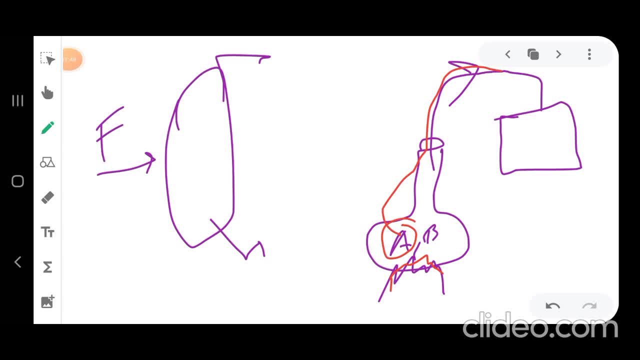 goes to the vapor phase, then you can add here a cooling system, for example cooling water or whatever, to condense this vapor and collect it here. okay, so it will mainly contains a and mainly a and some b, okay, and then after some time, from time one to time two, the end. 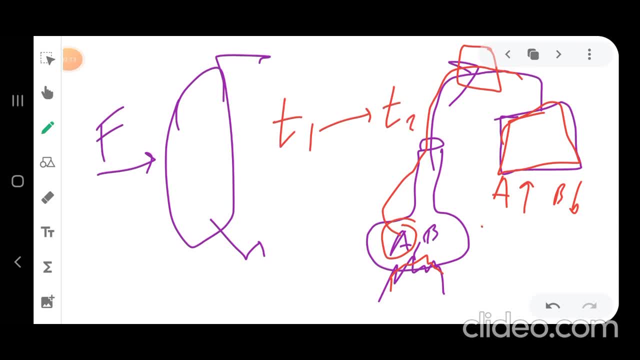 okay, after some time, you will left with a liquid quantity here that contains mainly b, the heavy component, and whatever you collect here will contains mainly a, so you separate them, you did your separation okay, again based on the difference in boiling point, which is the difference in volatility. okay, so, 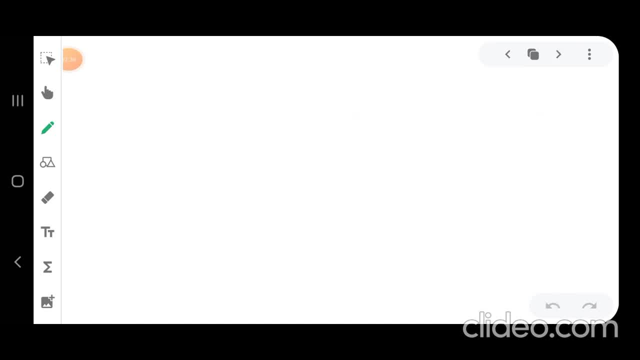 that's batch distillation. in batch distillation we we have mainly three modes, famous modes. we have three modes for batch distillation. the first mode is called simple, simple batch distillation, yeah, and the second mode? the second mode is called batch distillation with rectification. 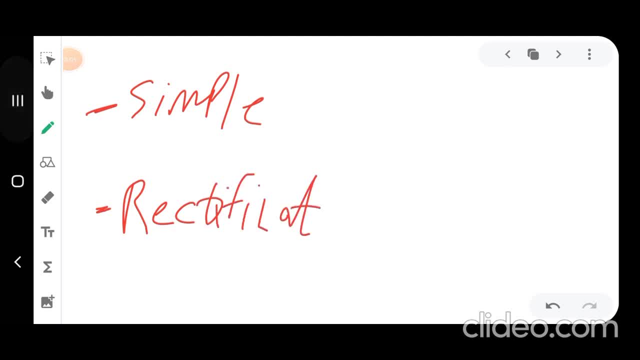 rectification, okay, and this mode, you can split it. so this mode, rectification, you can split it into two. we can have rectification at constant reflux ratio or or rectification with constant XD distillate composition of the more volatile component. we will talk. I will talk about all of these, but as a general idea, this: 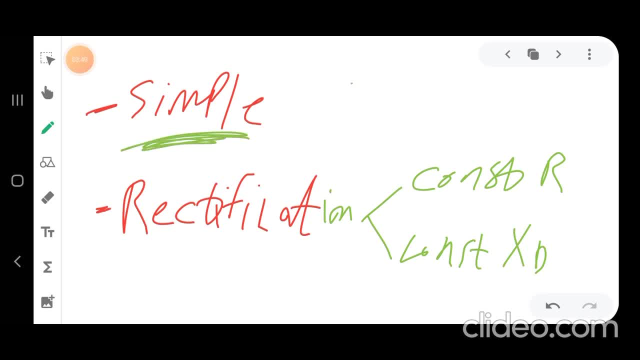 simple batch distillation, it is like single stage. so you have only this still pot and that's it. you have this still pot and then you collect your products here. but if you have a rectification, rectification it means that you have stages. you don't have like one stage here. the one stage is only the still pot. 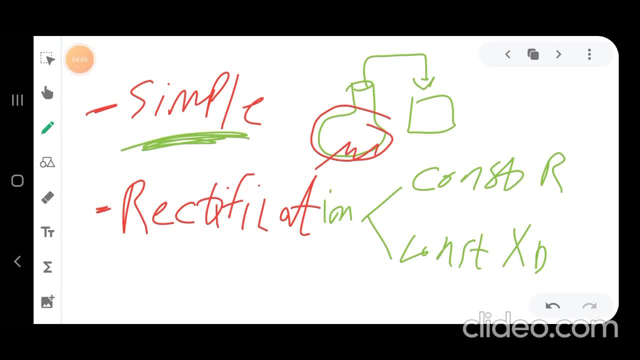 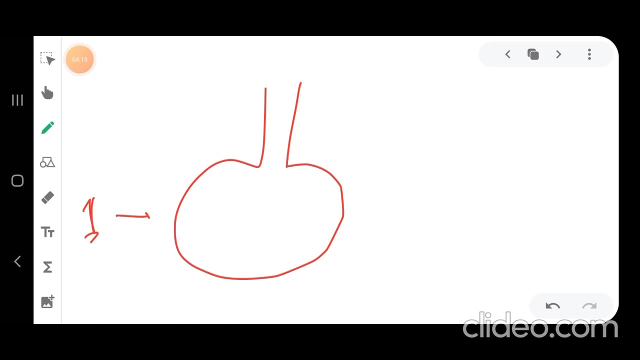 where the liquid is vaporizing. okay, but in rectification you use some equilibrium stages. for example, you attach them here like this: you have, this is the still pot. this is stage one, single stage, if you have only this. so this will be simple patch distillation if you have here. 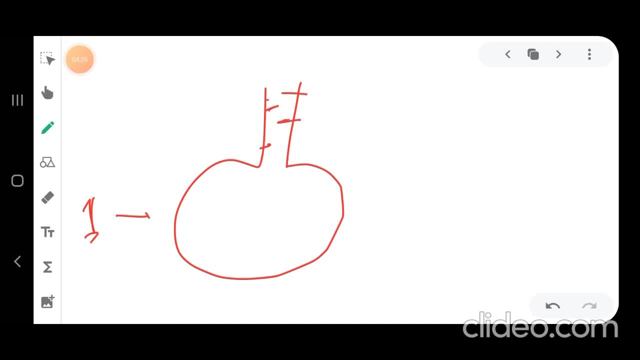 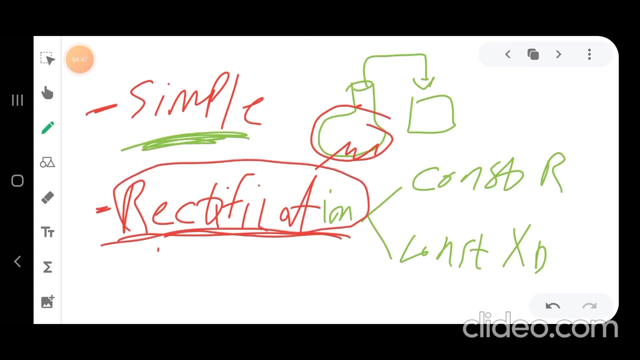 some stages, some stages, and then you take the product and you do some reflux. then you collect your product here then. so this is the reflux and you have here x decomposition of the distillate that you collect here. then this is called batch distillation with rectification. so rectification means addition of stages. you add some stages here. okay, if you add. 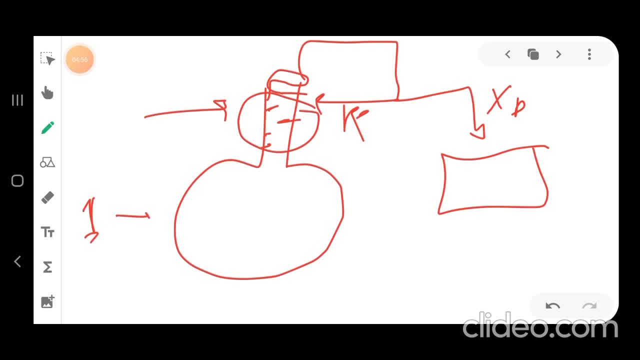 the stages and you use some reflux to maintain the continuous contact between liquid and vapor. this we call the patch distillation with rectification, and it has two modes. one mode is to operate constant r, so you fix this reflux, it it doesn't change. this reflux is fixed, so xd will be variable. 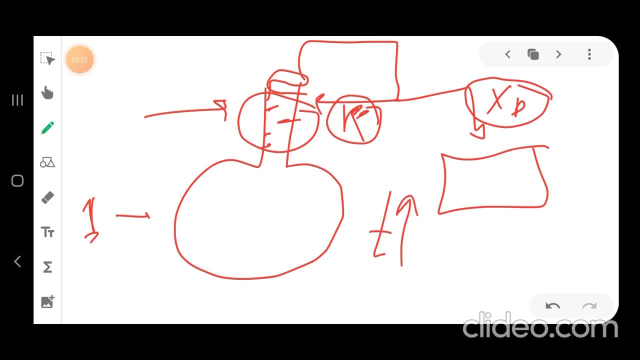 it's changing as the time proceeds. of course xd will change. okay, the distillate, or you have another mode. usually we do it through controllers. we need to use some controllers, which is not the scope discourse, it's the scope of control process. yeah, control process course. uh, use some control. 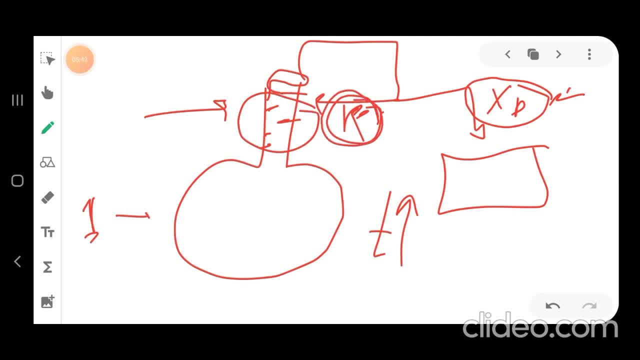 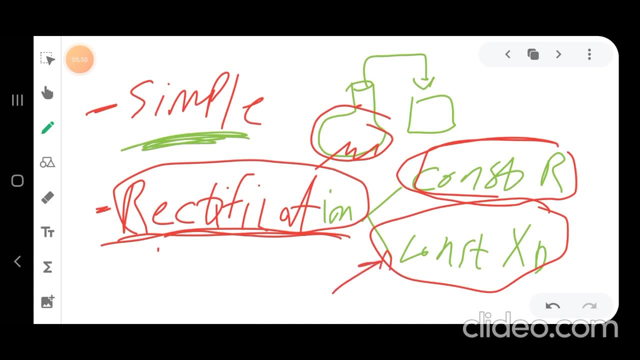 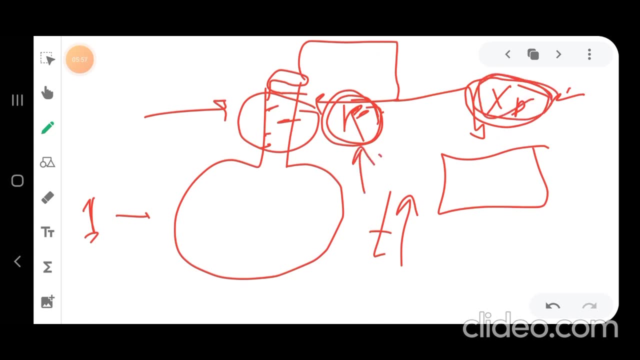 controllers in order to control this reflux ratio to be constant. this we call constant r, constant xd. it is somehow more difficult. you need to use some controllers in order to fix this composition and to do this you need to play with the reflux ratio. so the reflux ratio becomes. 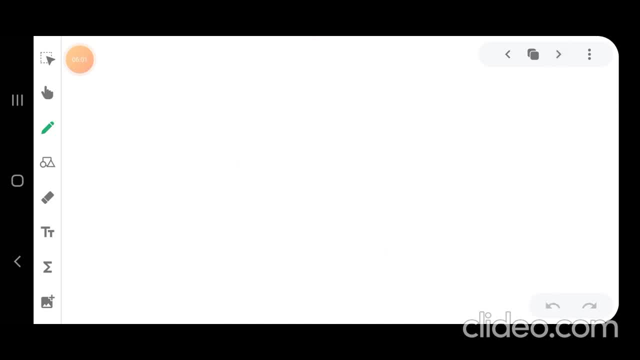 a variable. so let's discuss them one by one. first, we will start with a simple, simple batch distillation. but before i discuss the simple batch distillation, i want to mention something. yeah, i want to mention important something- that describing batch distillation, to describe batch distillation, we have an equation called batch distillation, in general, with a simple or 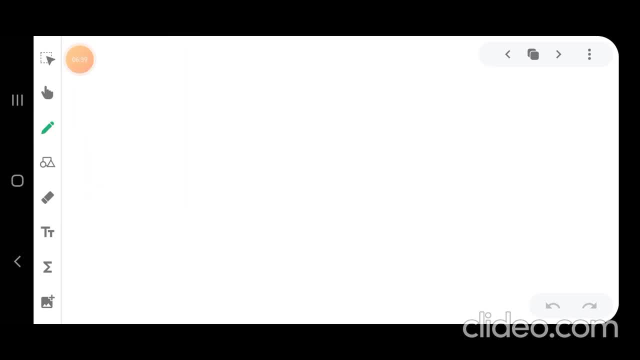 rectification. so batch distillation. in general we can use an equation called Rayleigh equation- Rayleigh equation for the scientist Rayleigh, which is a famous scientist, especially in heat transfer. i'm sure that you heard about this name before the Rayleigh equation, so this is Rayleigh. 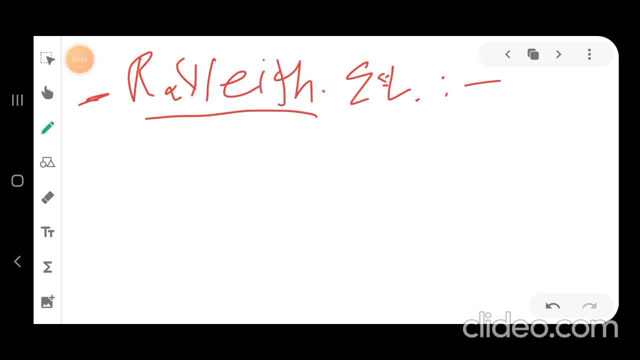 equation. Rayleigh equation is used to describe batch distillation with a simple or with a simple or rectification batch distillation. this equation tells you that len of w over w naught is equal to integration from x w naught to x w, dx w by y d minus x w. this is a general equation. okay, and what? 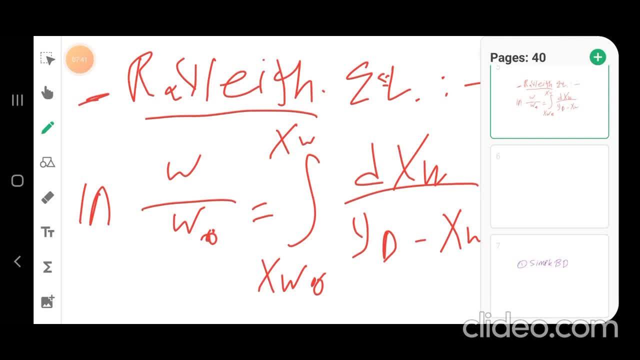 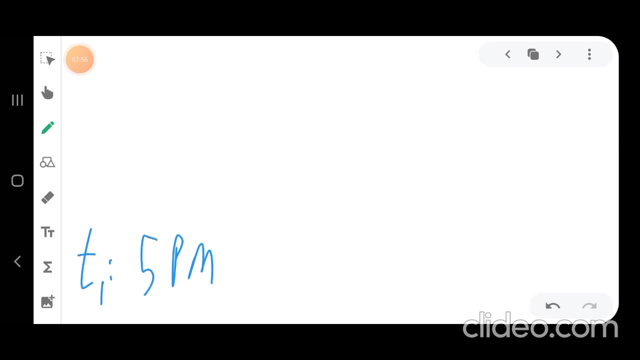 what i want to mention here is. what i want to mention here is: every equation has a story, and the story of this equation is: let's discuss it one by one. suppose we have a time, a time one, let's say it is 5 pm. then after some time, we have time two, after some time, which is, let's say, 6 pm, and i give him. 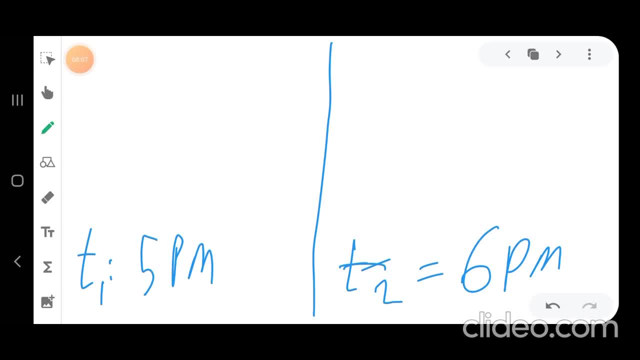 d n. okay, so we have here, this is our stillbot. okay, and we have the product here. we collect them into a vessel or a storage tank. okay, the initial amount of liquid presents here. initial amount of liquid presents here the mass of this liquid or the number of moles. another: 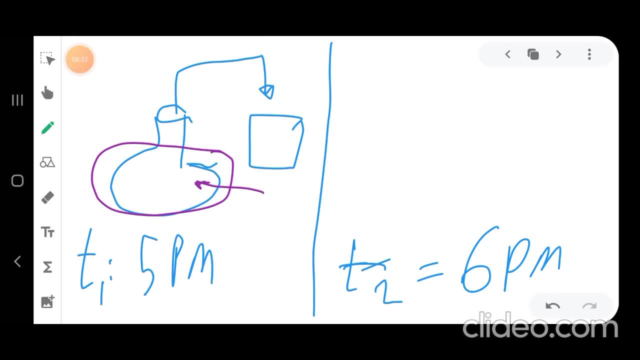 words and you can know the relation between mass and moles. it's just remodeled mass anyway, let's say the number of moles of this amount here initially at time one, and we refer always with time one as time zero. if you take this time as your reference, so you refer it to time zero. 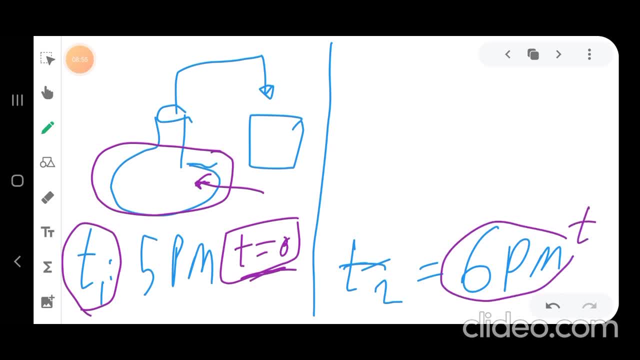 and then this: after some time, we call it time t. so from time 0 to some time t, okay, which is for our example. they are 5 pm and 6 pm, so in our example t is equal to 0. the initial time is 0. after some time which? 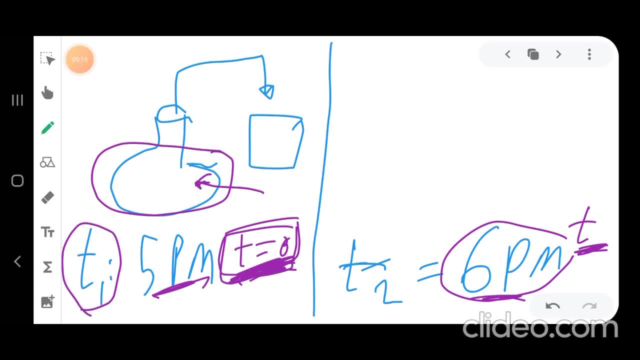 is one hour in this case we will have. this is the duration of the process. okay, so that the mass of, or the number of moles of, the liquid mixture. of course we have here a and b of this liquid mixture. we call it w0, so the w0. 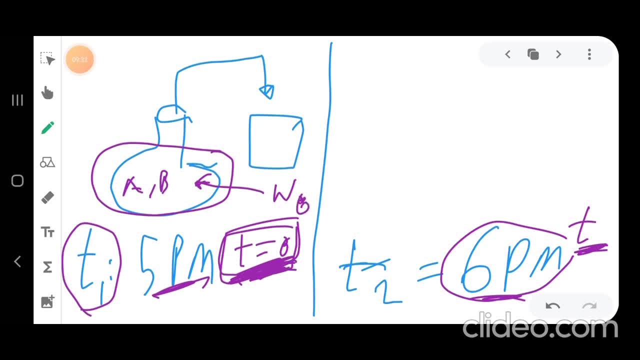 refers to the number of moles contained initially at time 0, then after some time, after some time. this is your stir pot. after some time, the. of course you are heating here. you use heat. okay, you are heating. so what's happening is that some amount of this liquid is vaporizing. so, as this vaporize, what will happen to? 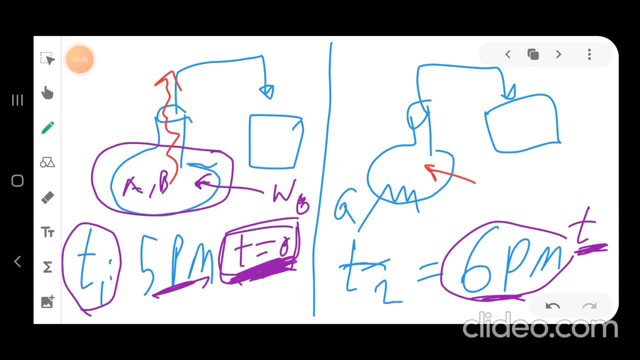 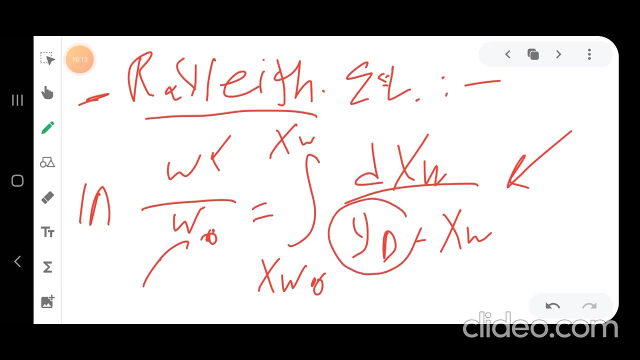 the quantity of the liquid. it will decrease, right? so the quantity or the number of moles of liquid that we left after the end of the process. we call it w. okay, so this is w and this is w0. okay, and then what's this? yd and xw- yd is the composition on the distillate and xw is the composition. 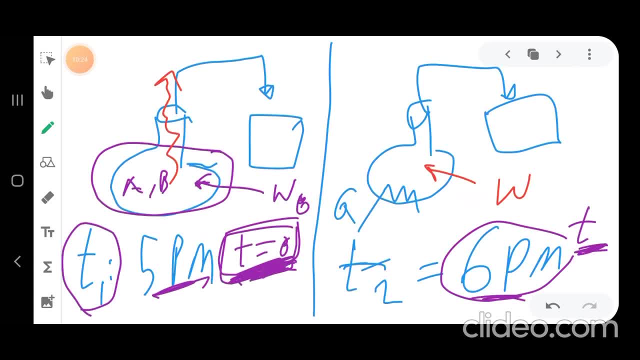 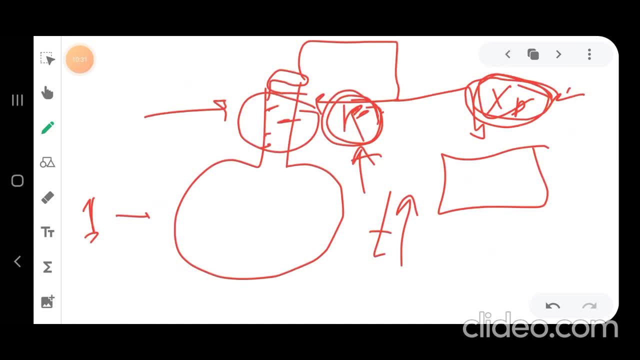 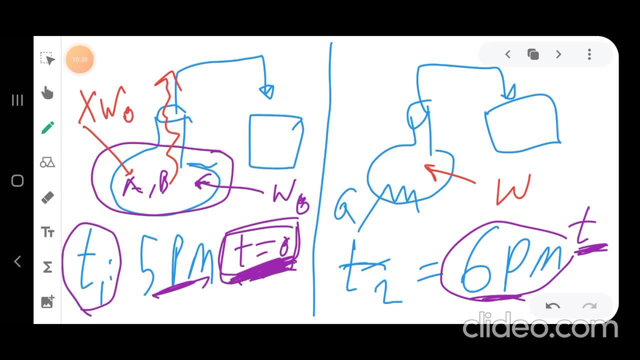 of the waste. oh, yeah, waste. so initially you know what do you mean by xw0, and w not refers to initially. so initially the concentration here, or the composition, is xw0, for a would be, of course, for the more volatile component, which is a for 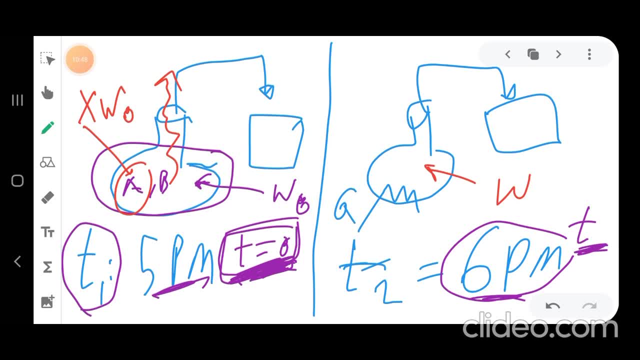 example, in this case, let's say, the more volatile component. so xw0 is the composition of a and the still both at time 0. after some time, this what will happen to this composition? we are heating, so the vapor will be generated, and as a is more volatile, so more a will be collected more. 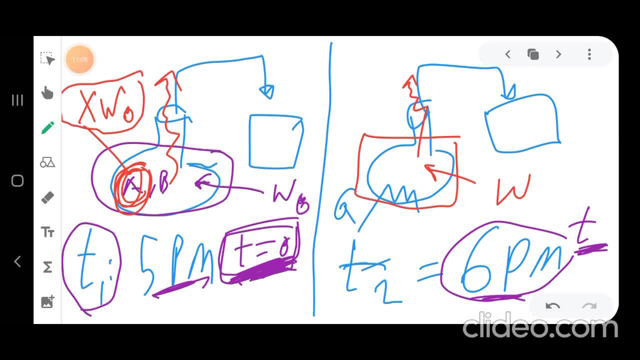 a will leave this still pot. so of course xw will decrease. so the composition of the a: after some time we call it xw and of course always xw will be less than xw0 because we are vaporizing. okay, so this is xw and this is xw0. yd is same as xd, xw0 is the same as. 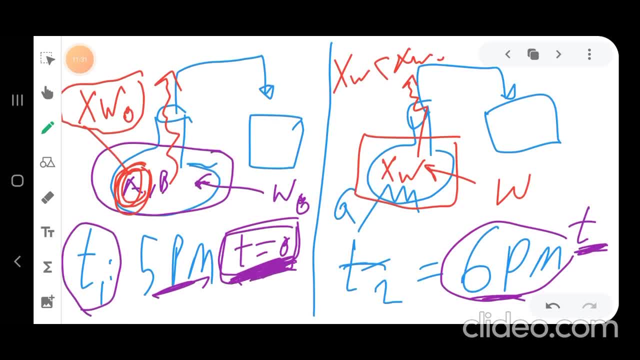 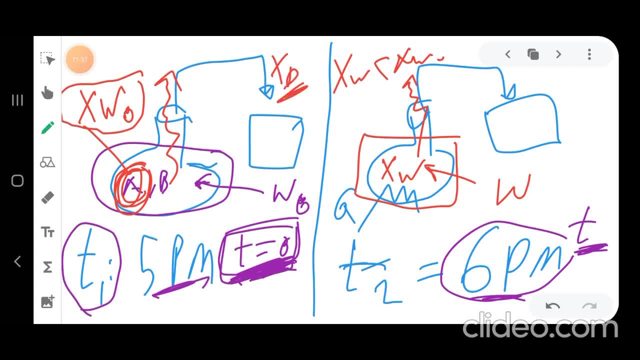 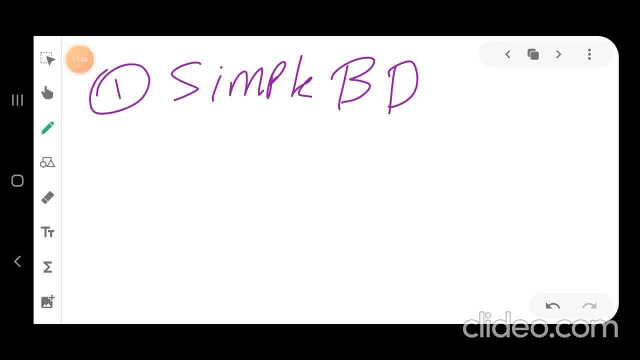 the distillate here xd or yd? okay, yeah, that's a Rayleigh equation. so now let's start with the simple batch distillation. simple batch distillation, the simple batch distillation, in other words, in simple patch distillation we don't have reflux, we don't have stages, we don't have this complexity. that's why we can see. 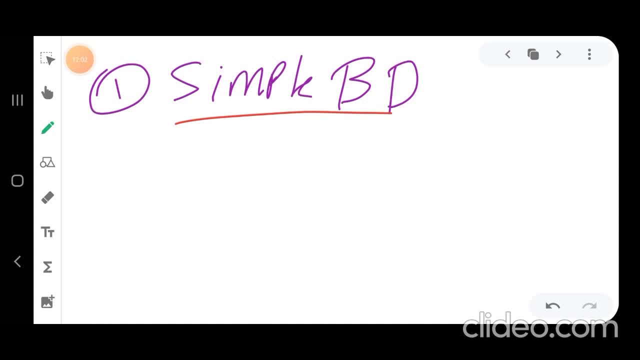 that we can say that the distillation composite, the distillate composition, is nothing but the composition in the vapor phase, because we have only single stage. and we can say also that composition in the still pot xw is just the composition in the liquid, because we have one. 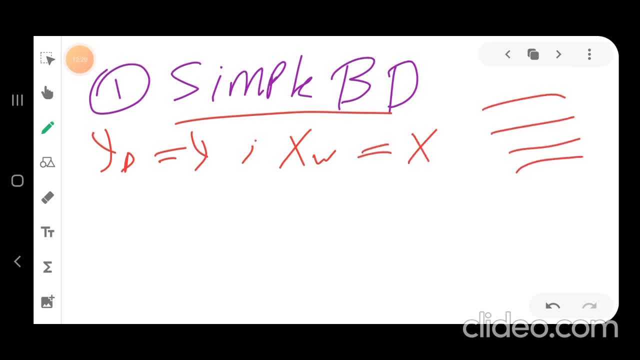 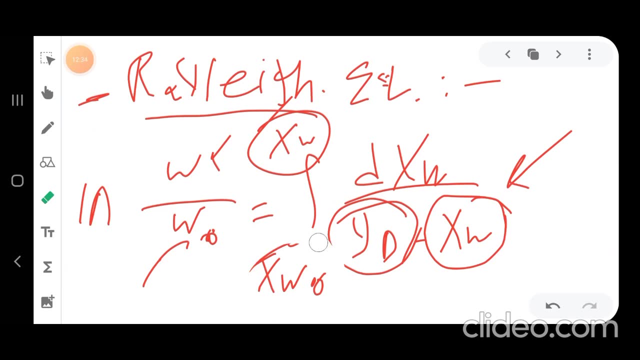 stage. we don't have that too much stages and each stage we have it is on x and w, x and w. no, no, it's just a single stage. that's why we can use this and then see this really equation: we replace xw, not with x. not, we replace xw with x and we replace the x. we replace the xw with x, y, d with y, xw with. 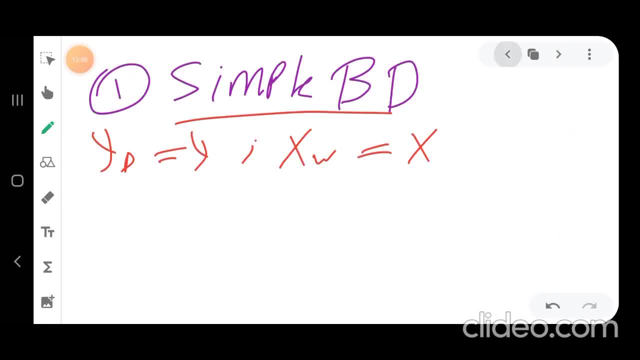 x, so we were left with this equation. this equation is only valid for that. i'm going to write now. this equation is only valid for simple batch distillation, which is the sorry. then. w over w not, is equal to integration from x, not the initial composition in the liquid phase up to x. 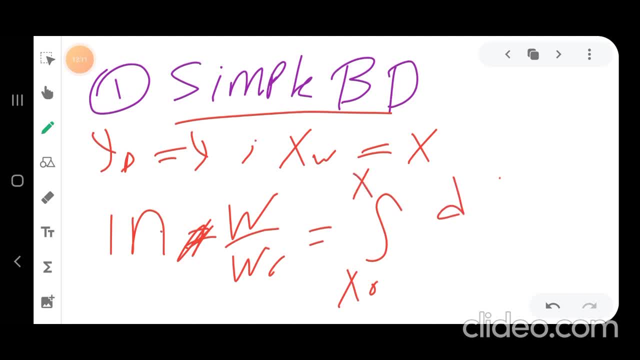 the final composition in the liquid phase: dx over 1 y minus x. yeah, that's it. this is the equation. derive it from where? from the Rayleigh equation. and the Rayleigh equation is derived from where. it is derived from a simple material balance, using honestly the state process: material balance, more balance around the still pot. okay, so that's it. this is the. 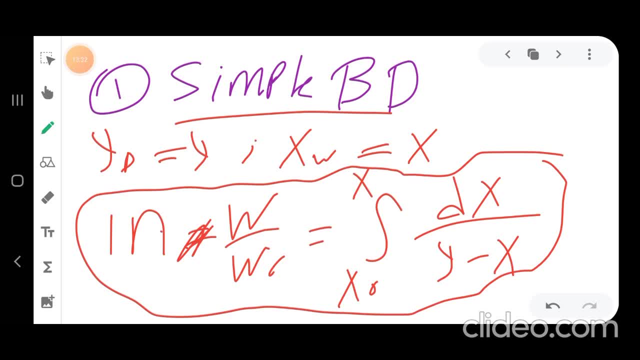 equation for the batch distillation. now the problem here is how to find, for example, if you are interested to know, if we are interested to know, the quantity that we left with, which is w, after some time. if we know the initial quantity, w not. the problem here is how to calculate this. 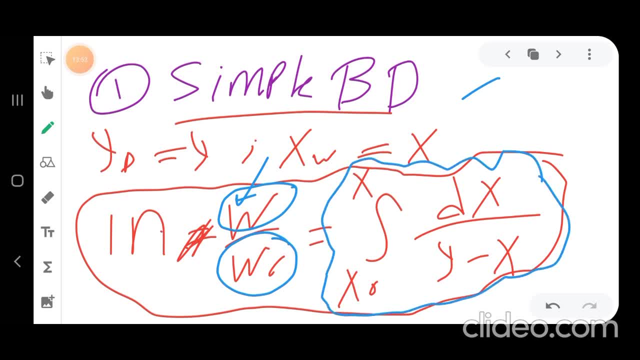 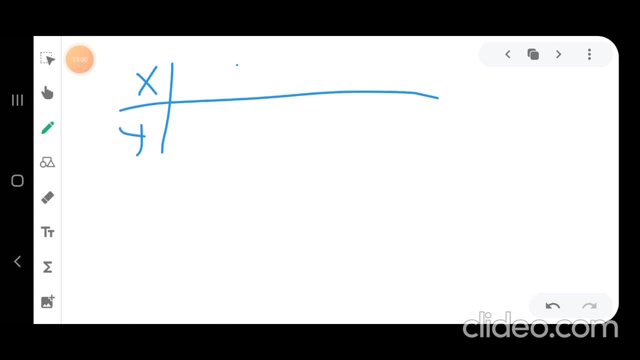 integration. how to calculate this integration? we can have three ways. the first way is: if we have a table that contains x and y values, the equilibrium data, then what we do? we use a numerical integration. we use a numerical integration. so how to integrate this integration? of dx, y minus x, we have integration of 1 over y. 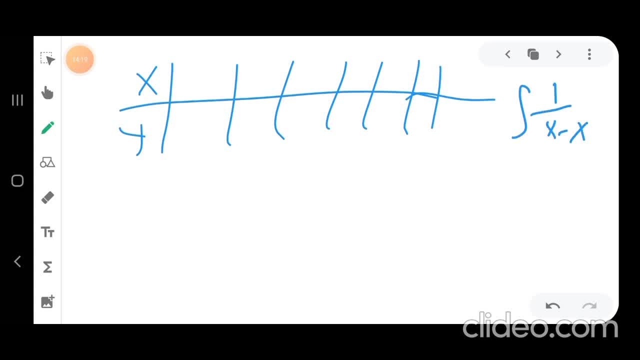 minus x, integration of y minus x- dx. so what's our f of x here? what's our f of x? this is f of x, this is our f of x, right? so this is our f of x. so, in order to integrate what we will do, we'll do a table same as numerical. 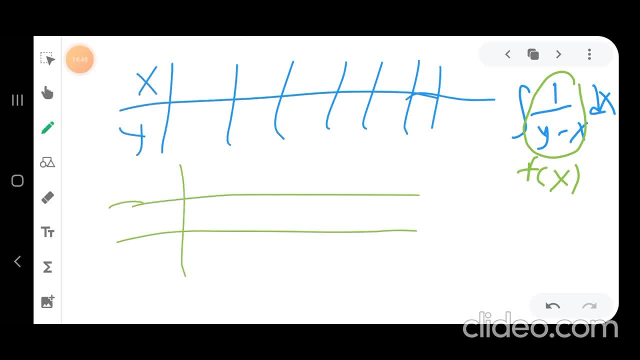 table to do numerical integration, then the first thing is to to have this x, starting from x, naught to the end. okay, the initial composition of the liquid phase. of course we refer to composition, as always, to the more volatile component. okay, then we have these values of y. 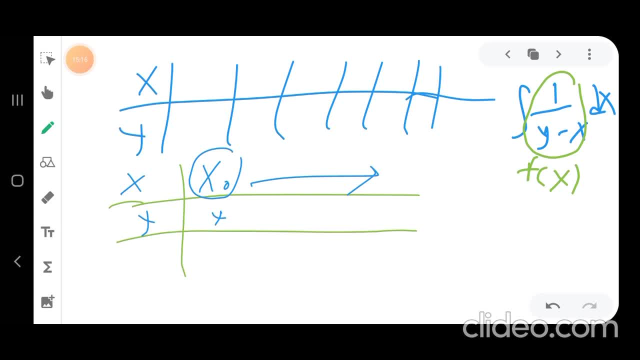 have these values of y, starting from y, naught at the end, then what we will do? we just find f of x. as simple as this. f of x will be 1 over y minus x. you find 1 over y minus x for this, then, for all values, then you do numerical integration. 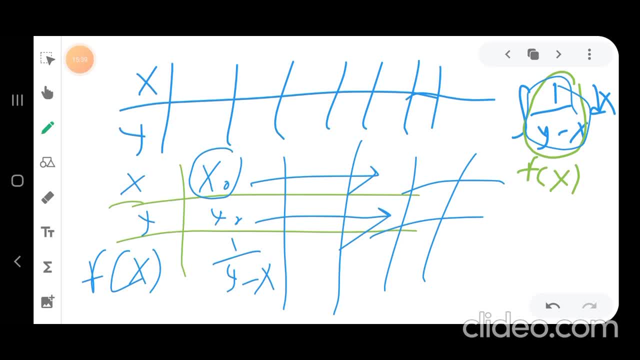 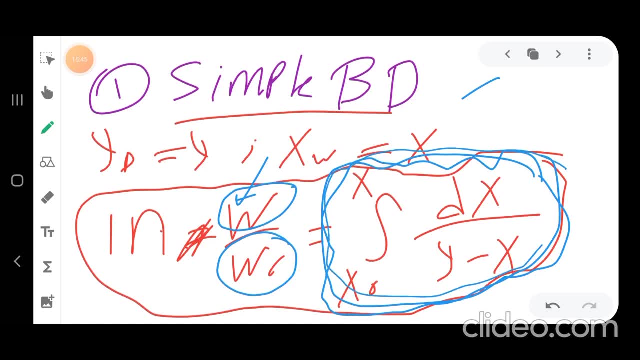 one of the ways is to use trapezoidal rule. so if you want to find integration, this one, only this part, only this part. in other words, we can say: integration, only this part of the training. another word: we can see: ln, w over w, not equal to i, integration. how to find this integration one? 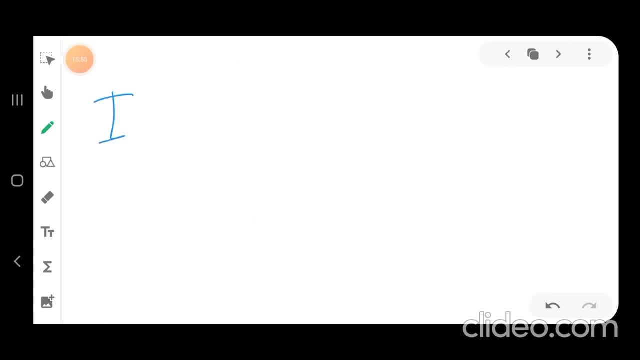 of the ways, easiest ways, to apply a trapezoidal rule, or you can use simpson 1 by 3 rule, simpson 3 by 8 rule, quadrature rule or whatever new american method, but the easiest way is the trapezoidal rule. yet enough for design calculation. and this integration is just. they find it as h. 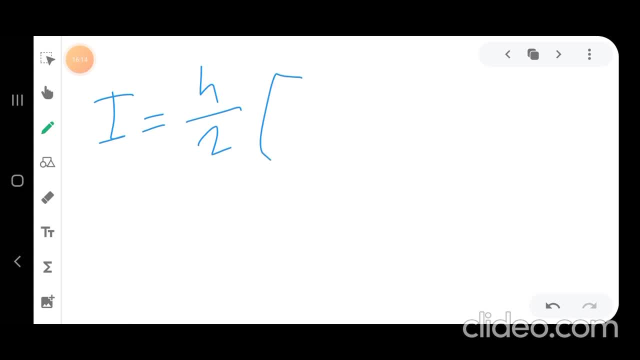 over 2, if i'm not mistaken, then you find f naught plus 2, f1 plus etc. plus 2 f n minus 1 plus f n. so it is like if you have, for example, five points, if you have five points, then it would be f1 plus. 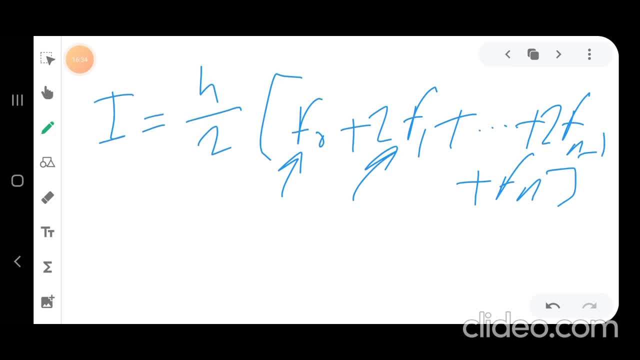 2, f2 plus 2, f1 plus 2, f3 plus 2, f4 plus f5. so in between you multiply, you multiply each f by two at the beginning and at the end. you don't have to do this. okay, let's start by. 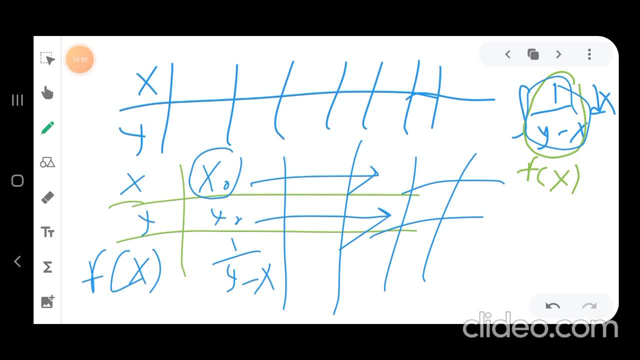 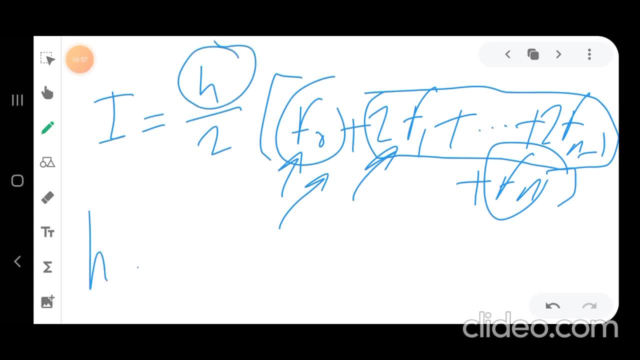 the trapezoidal rule. so that's why we make this table. in order to find f of x at different points, then we use this rule. and what's this? h? h is just p minus a over n. okay, so if n is the number of intervals, be careful here- n is number of intervals, it's not the number of points. it's like if you. 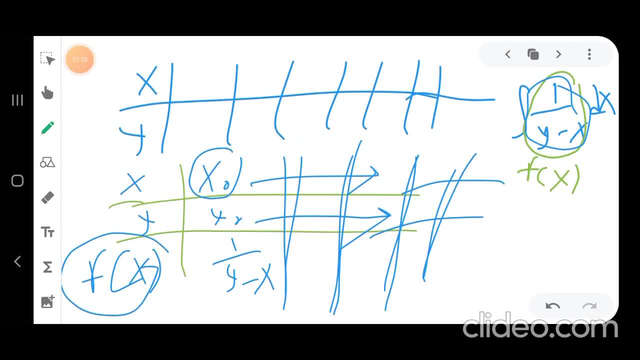 have five points, like here: method one, two, three, four, five, six, seven. let's say seven point how many intervals we have. they will be number of points minus one. how? because from here to here is one interval: two, three, four, five, six, six intervals. so this n is not number of points, it's number of intervals, which is number of points minus one. 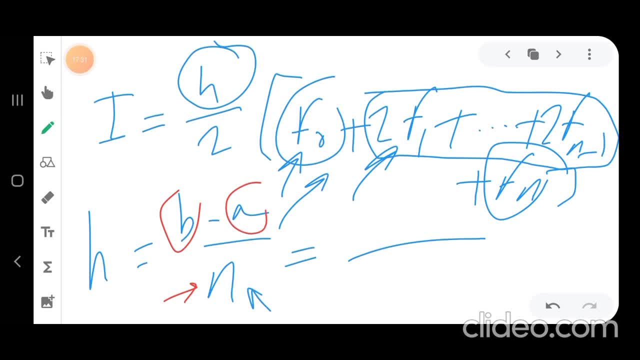 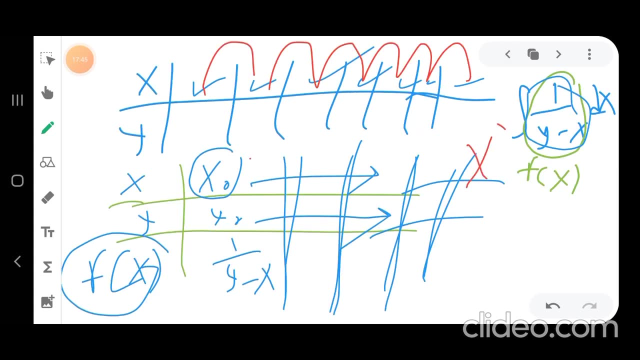 okay, and what's this? p and a? p is the final component, p is the is the final composition of the liquid phase. a is the initial composition in the liquid phase divided by p. okay, so the, the final value of x minus the initial value divided by the number of intervals. 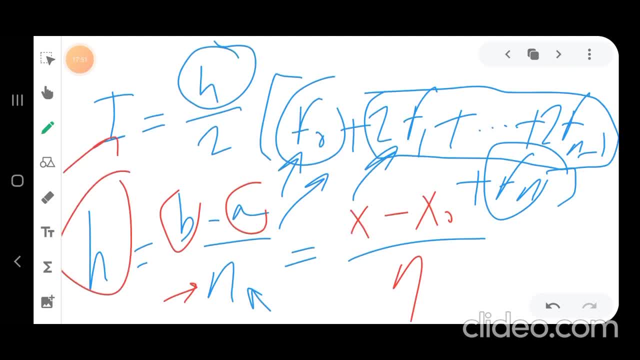 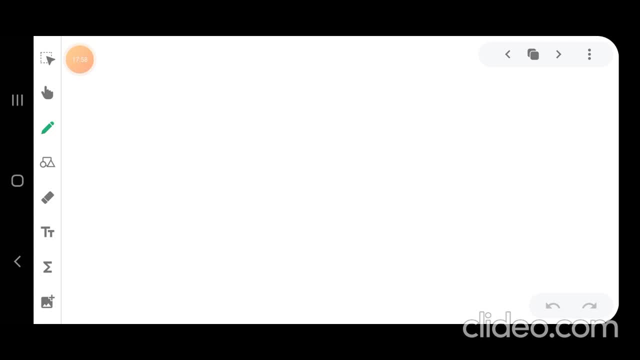 you can give this h, then you can get this integral integration. and of course we are not interested only in the integration we at the end of the day we want to find w the quantity of the liquid that we left with. so we can say then w over w naught is equal to this integration, or in other words, 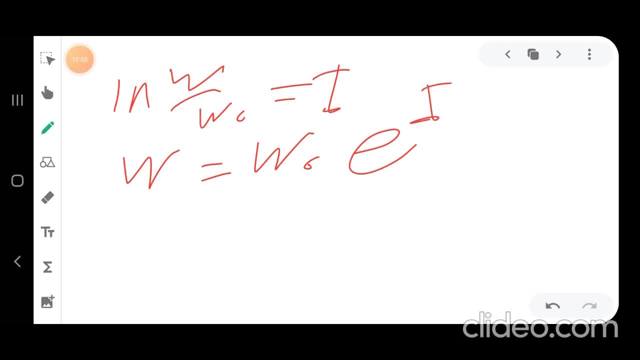 w is equal to w naught e to the power integration. if you have integration, you know initial quantity, you can get w easy. okay, that's it. and we have some special cases, like special cases of this equation. the first special case is if you have a constant for constant k distribution coefficient and you 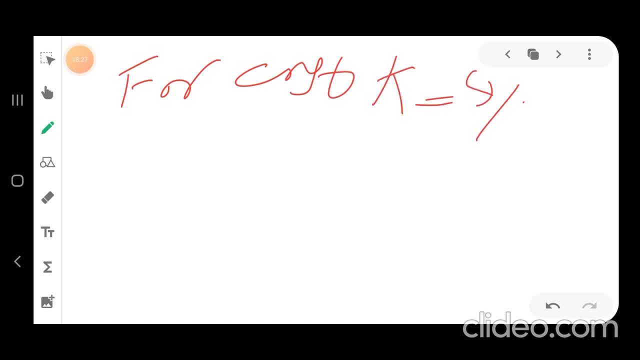 know this distribution coefficient is y by x distribution coefficient. if you have this constant, then you can use analytical integration. you will substitute with: y is equal to kx. okay, then you can integrate the equation analytically. you don't have to use a numerical integration integration. then you will left with this equation: in w over w, naught is equal to. 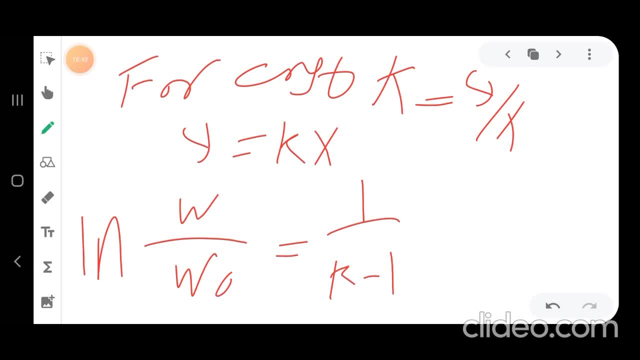 1 over k minus 1 the distribution coefficient, then x over x. you can try this integration. this is just the integration of the Rayleigh equation, substituting y with kx. okay, the third special case is what if you have a constant for constant for constant relative volatility? 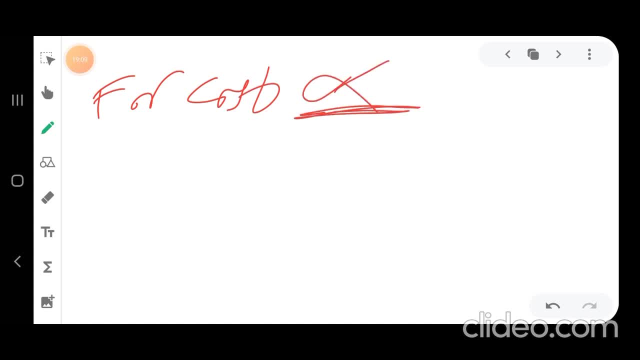 alpha. if you have a constant relative volatility and this assumption looks valid, then what you have to do is you again integrate the equation analytically. it's somehow difficult to integrate, but if you have time and you try this integration, you will left with this analytical integration. then w0 over w equal to 1. 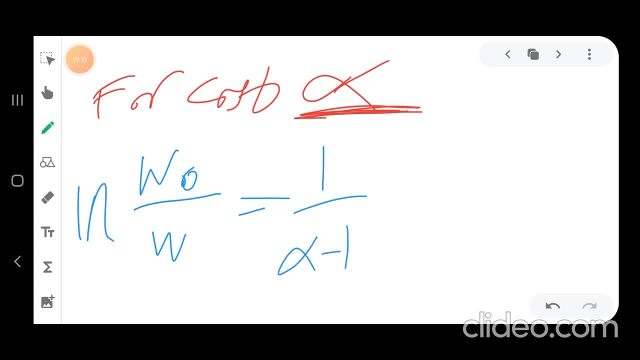 over alpha minus 1. then we have len x0 over x plus alpha len 1 minus x over 1 minus x0. yeah, that's it. this is the analytical equation, and you be careful that it's only valid if you have a constant relativity, if you have a. 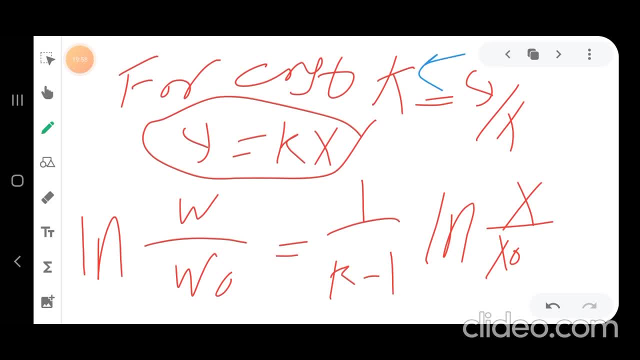 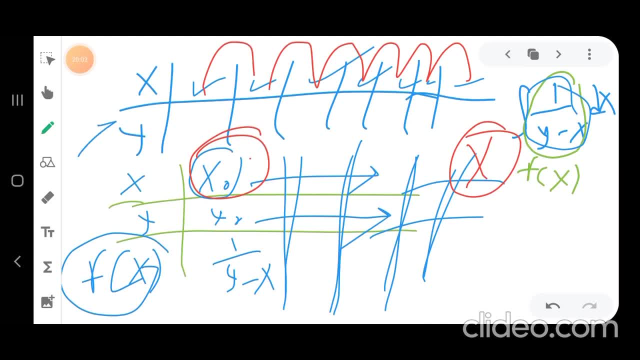 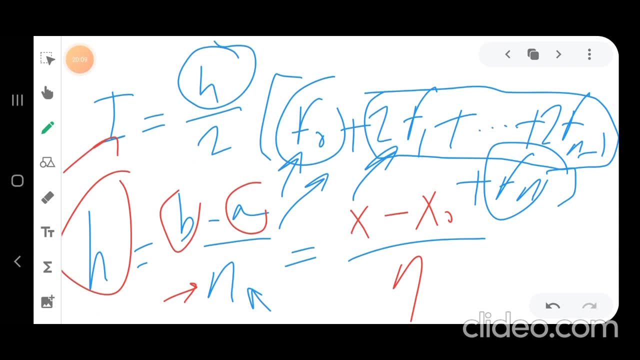 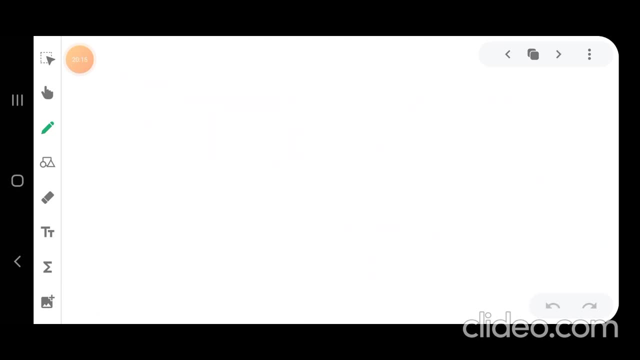 constant alpha or constant k. you have a table. then you need to go for trapezoidal rule and integrate this equation analytically, numerically, numerical integration, trapezoidal rule or whatever rule- okay, and there is a good equation to discuss using material balance. you have this right. you have this. 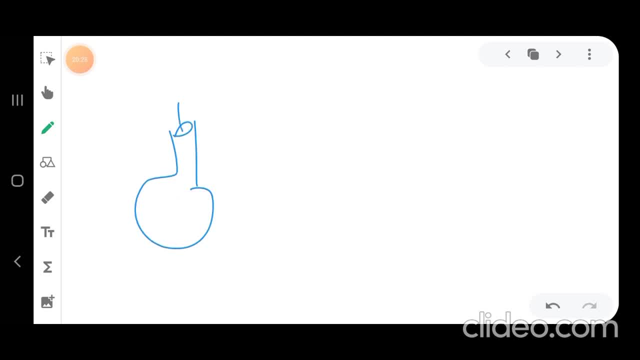 your still pot and then you collect the sample here, you collect your product here. okay, so let's do a material balance. if you do material balance around this table so you can see that the initial quantity w0, initial quantity here- is equal to. after some time you will left with some quantity w and, of course, this: 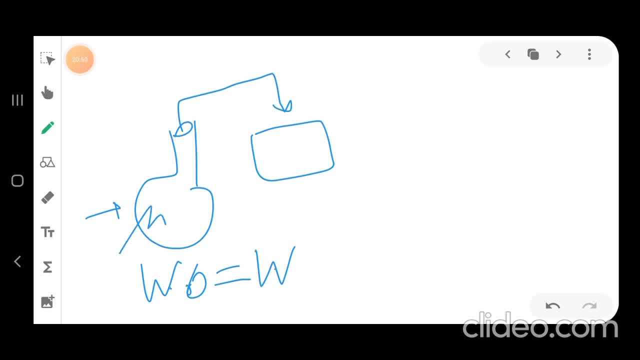 w is less than w0 because you are vaporizing, okay. so of course, this w0 will be summation of the left quantity after vaporization, after the process finished, finished, plus something called d total. what do you mean by d total? d total is the total amount that you collect here, which is a logical equation, logical. 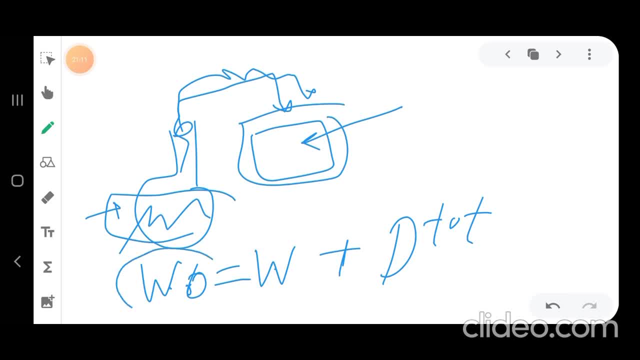 equation: yeah, if you start with a specific quantity w0, after some time you will get some quantity left here and some quantity collected here. we call this d total, the total quantity collect. so it is not a read, it is not like mol per time second. no, no, no, it's just quantity mol, because we are dealing with batch, not 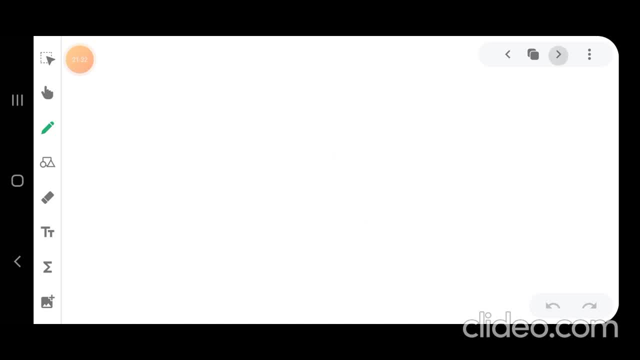 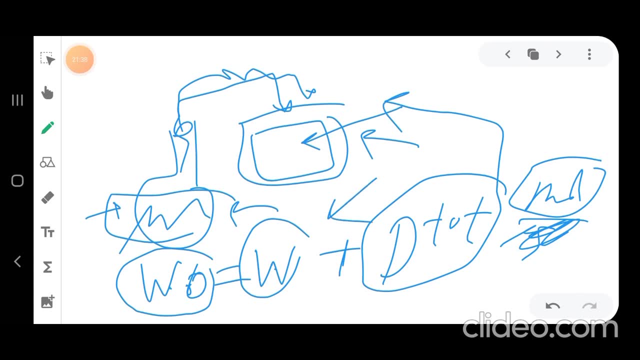 continuous. okay, so this is it. also, this is for the overall. if you do overall material balance, if you do component material balance, it is like you multiply by the composition, each side, so you will get this equation. you have this. you know this equation right. w naught plus d total. 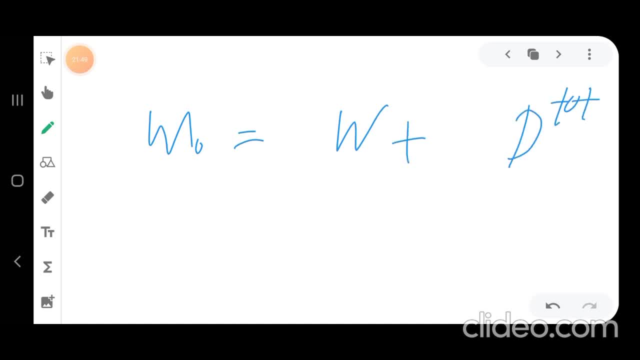 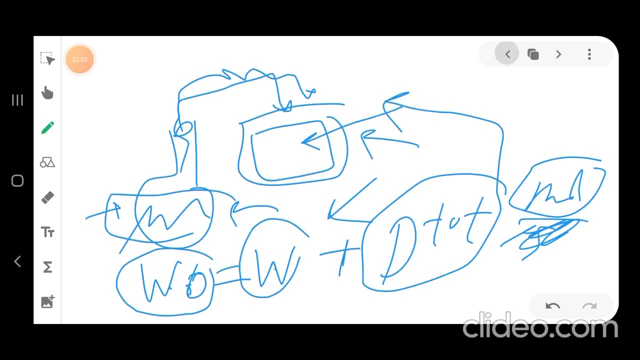 now let's multiply by so, in other words, we are doing material balance for components. so it will be x w naught, x w, then xd. but the problem here, a very important problem that i would like to discuss, is that there's a problem here. is that this xd? it varies with time as you vaporize? 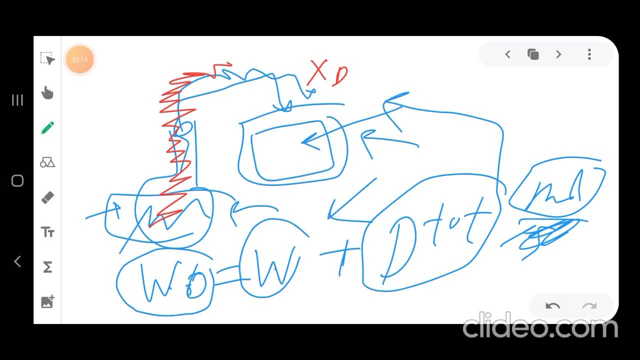 as you vaporize, you will take more b with you, isn't it? and b is a heavy. but as you vaporize you are giving more heat, so you are initiating this heavy component to b also vaporize it. so what will happen to this xd, which is the composition of a? it will decrease. 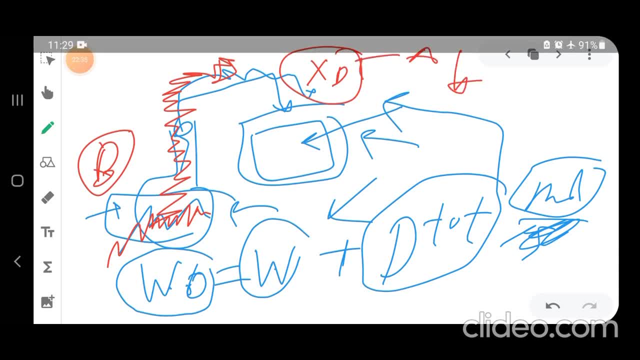 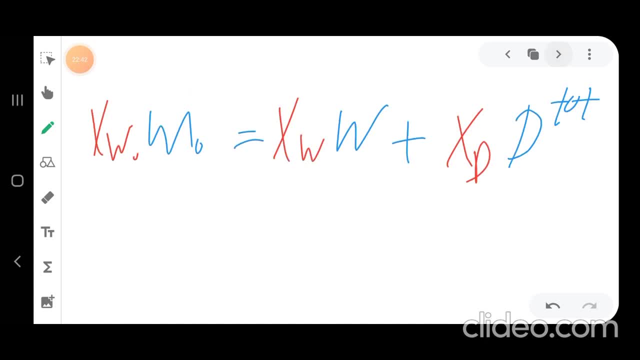 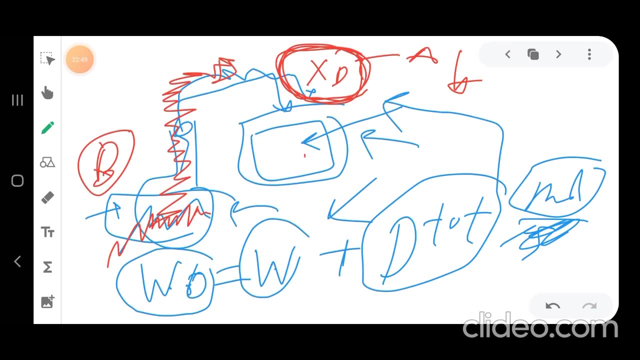 okay, so you will don't. you don't have this constant xd in simplified distillation. that's why we feel the need to use the average value. and the average value how to measure it? simply, you take a sample here. you take a sample here from this product, you analyze it in the lab and get 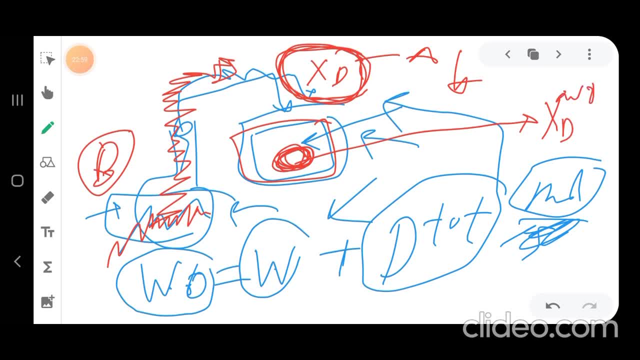 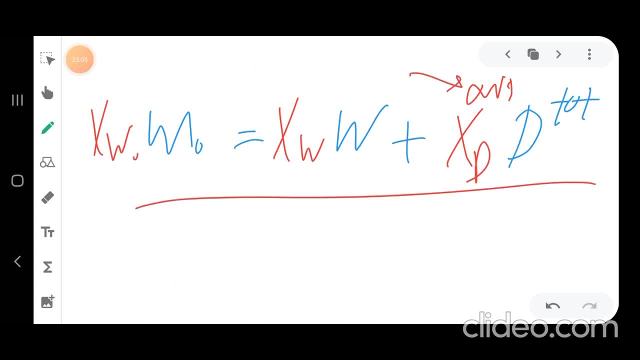 xd average, which is the average, the composition of the morbid tile component. that's why we use average. okay, okay, that's it. uh, yeah, okay, suppose, if we are interested to calculate the time of this distillation, how much time we need to wait in order to get this degree of separation for distillation. so the 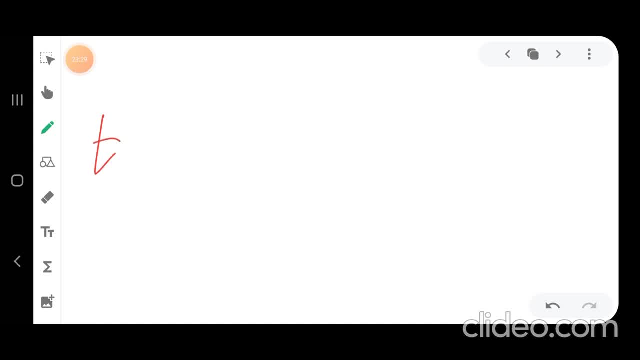 but it can be calculated through using this equation: time as d total, the total quantity that we collect over the d. d refers to the rate. the rate why? because you know we have this still, but it is like i like to say that it is not batch, it is semi-batch. why? because you don't have you. 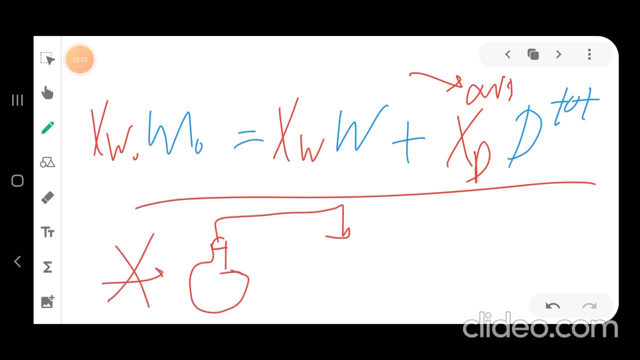 don't have continuous inlet but you have a continuous outlet and then you collect this outlet here. the amount that you collect here will refer to d total total amount. but as the time proceeds there is some rate here, some continuous product. it is like semi-batch process, but it is. 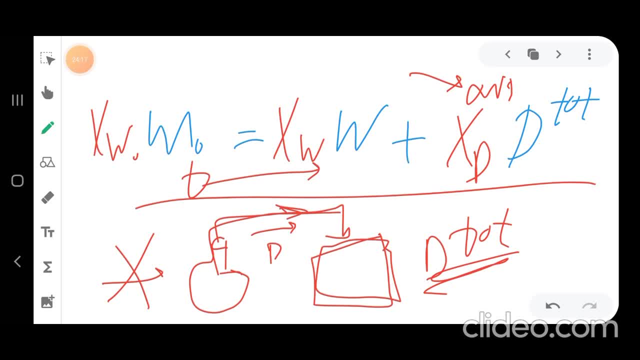 under the umbrella of the batch distillation. okay, anyway, for this rate here, this rate, this the flow rate of vapor leaving the still pot. we call it d d total if it's the total quantity that you collected at the end of the day. if you divide them, of course, this has a unit of 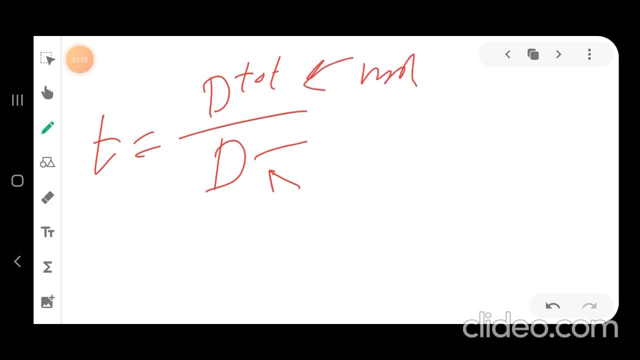 mole or kilo mole. this has a unit of mole per time, let's say more per second. if you divide them, you get unit of time. this is the time required for distillation. okay, this is the time required for this ratio and, by the way, this equation is not only valid for this. 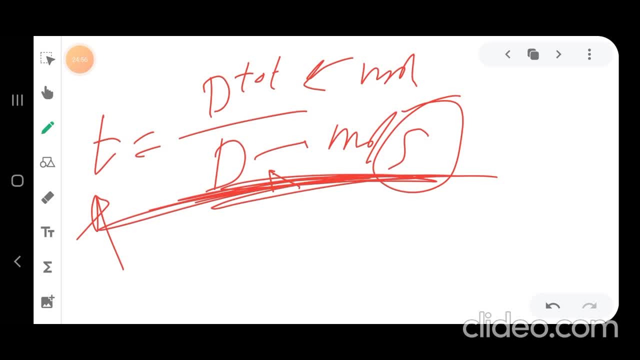 equation only. this equation is not valid only for simple distillation. it can be used also in batch distillation with rectification, but be sure that this g is constant if this d is varying. if it is not constant, then you cannot use this equation and we will see we are going to use another. 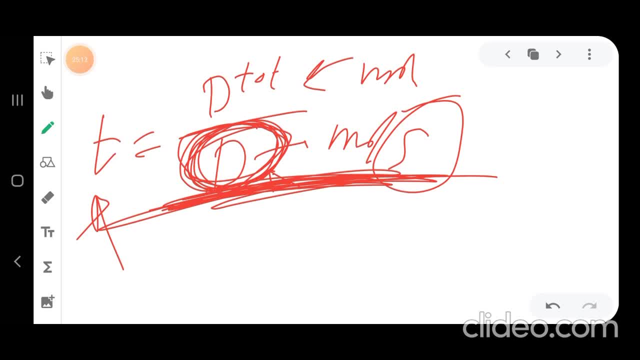 equation: if we have a constant, if we don't, if we don't have constant distillate rate, we need somehow integration to get the time okay. and you can know, this equation can be written in this form: w naught minus w over d. from where we get this? because we know from material balance d total is. 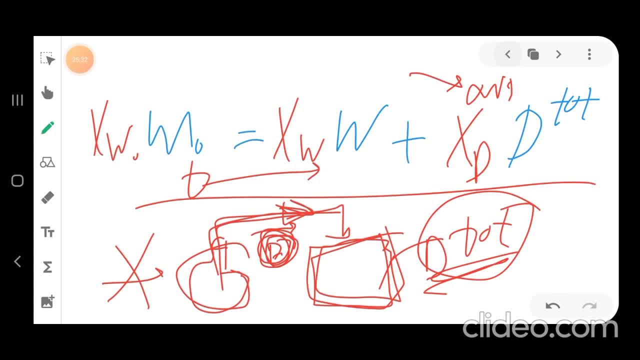 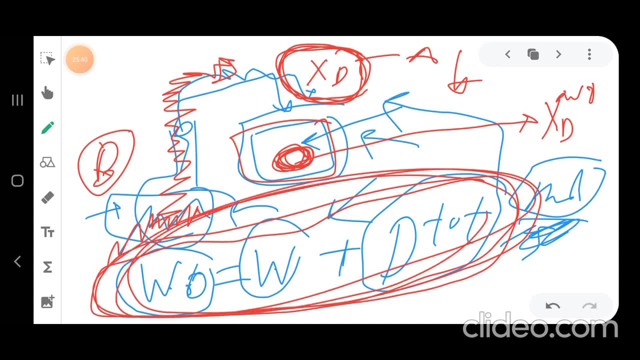 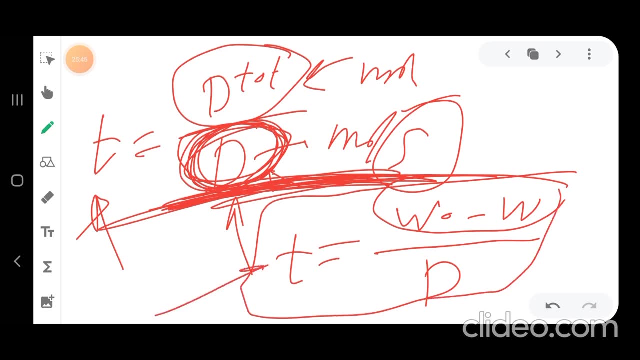 w naught minus w here, right, we discuss it. this one w naught is equal to w plus d total. so d total is w naught minus w. so you can get this final equation that you can use in order to get the time for any batch distillation with a simple batch or batch with rectification. okay, but 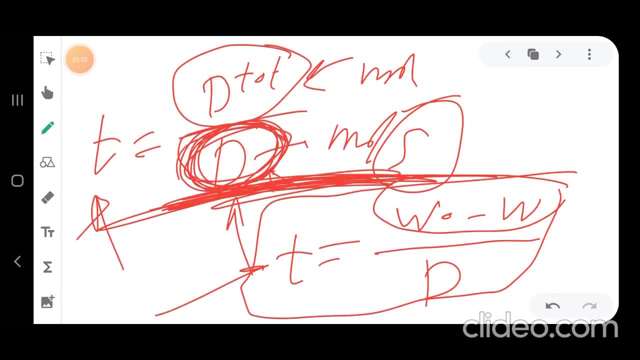 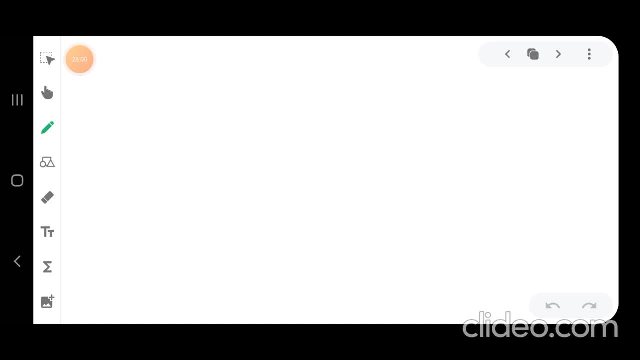 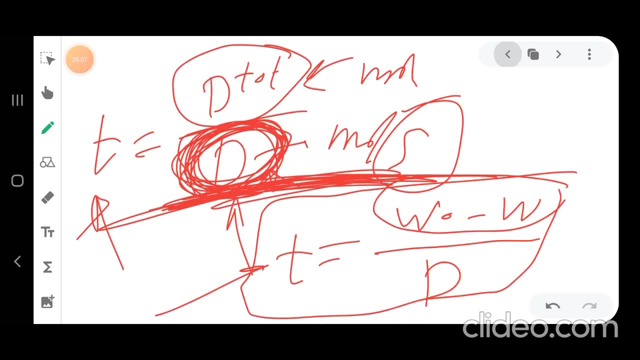 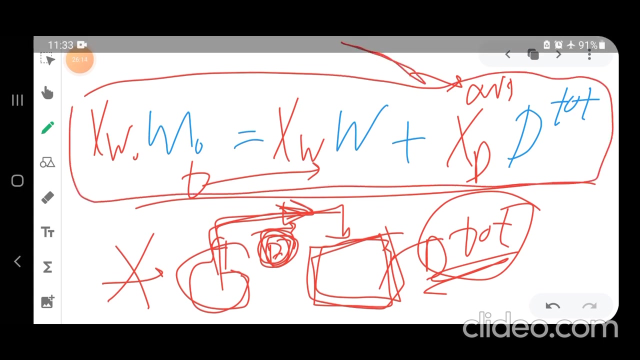 provided that this d is constant. okay. what else? okay, and already we discussed this equation. right, this equation? we discussed, it suppose. if you are interested to calculate, rather than going to the lab and take a sample and measure xd average using an analytical chemistry technique like spectroscopy or whatever technique you use instead of knowing all of this, can we? 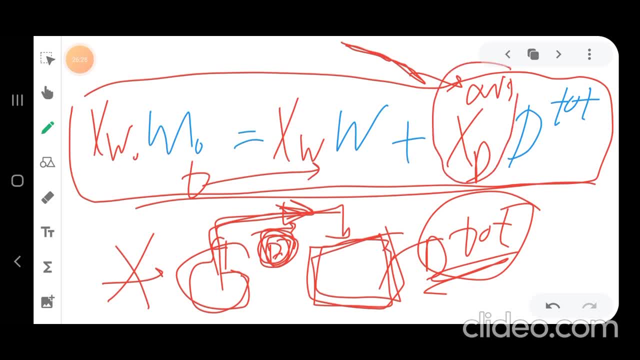 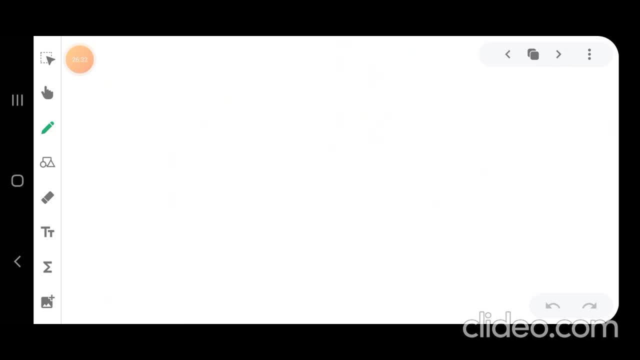 calculate this xd average? yeah, we can if we rearrange this equation in terms of xd average. just try to rearrange this equation, you will get this equation, xd average. and this is if you are interested to calculate the average composition of the distillate and the product. 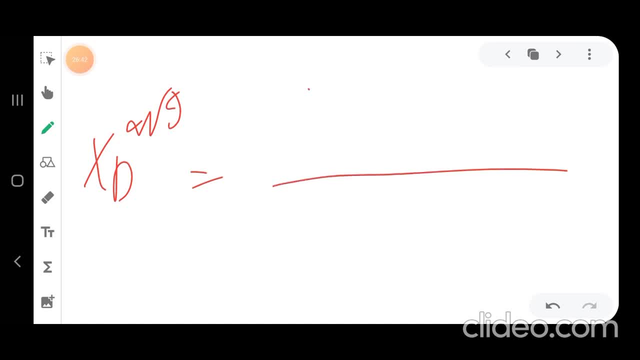 that we collect. if you rearrange it, you will get it as this: x w naught minus w. naught minus x w multiplied by w over w naught minus w. that's it. this is if you want to get this d average. okay, regarding there's a point that we would like to mention, it's regarding numerical integration. 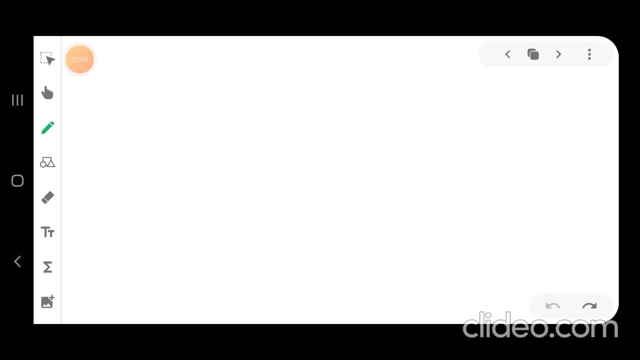 a problem that we face in a numerical integration is that we don't have an, an equal intervals. and if you have this x and w, if you have here 0.5, then 0.4, then 0.3, then 0.2, then you can see, here somehow we have a. 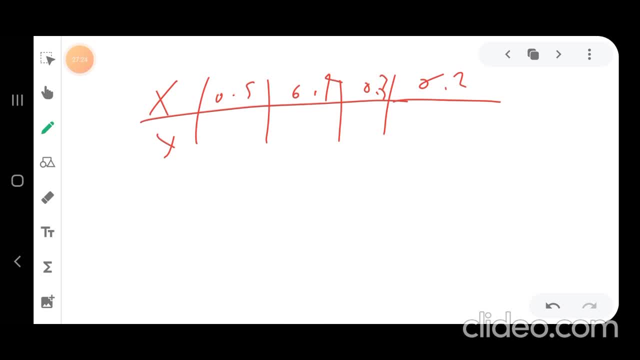 correlation constant interval, which is plus, not plus minus 0.1. this is our h interval. we move minus 0.1, 0.5, minus 0.1, 0.4, then 0.3, 0.2. then in this case we can use that repository that we already discussed. 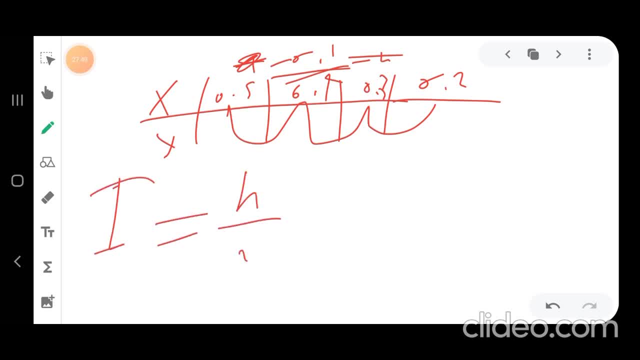 which is h over 2, f0 plus 2 f1, etc. up to fn. we have already discussed this. okay, but the problem here: what if we have unequal intervals? what if we have unequal interval? we have, for example, something like this: x and y, then we have 0.5, then 0.45, then 0.31, etc. whatever. so you can see, we 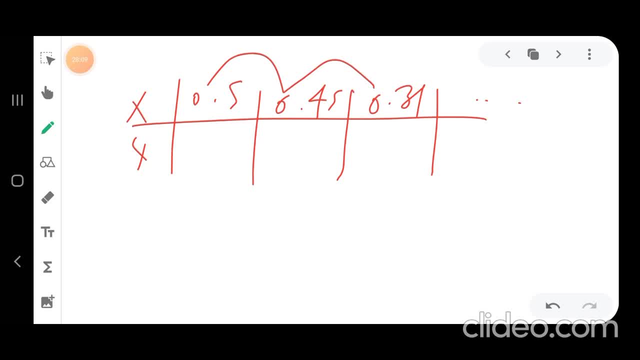 don't have a constant interval. so this case we call it unequal intervals. and is there a solution for this case? yes, there is. we can apply again a modified form of trouble. the rule that's in this one, i, the integration, is equal to summation of x, i minus x. i minus 1. 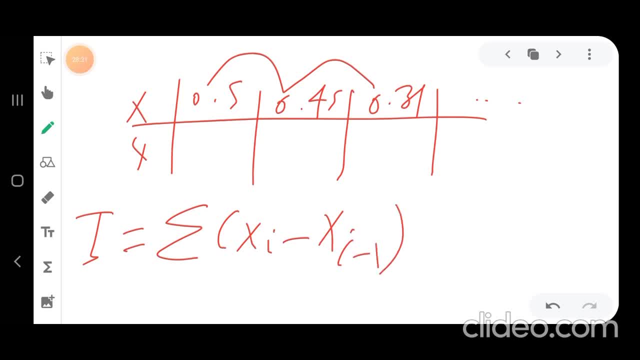 multiplied by f of x i minus 1, plus f of x i divided by 2. what we are doing here? suppose we have only three points, then what we will do, we will say this will be: x i here will be 0.45. x i minus 1 will be 0.5. f of x i minus 1 will be the value of f. remember. 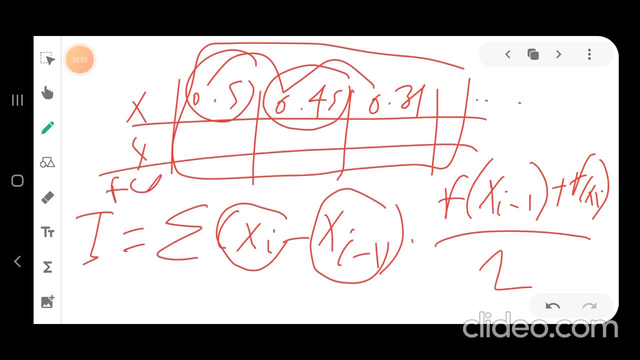 when we calculate f of x, the value of f at x, i minus 1, and at this point this will be f of x- i minus 1, then f of x- i will be the value of f of x at this point. okay, then it is summation, so you: 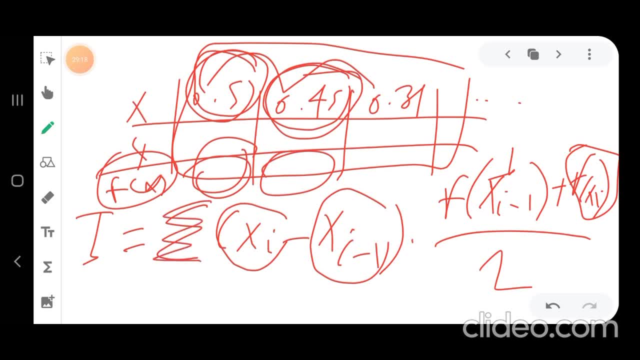 need to continue. continue, then plus. you take a plus, then continue this. you will. let me do it in a different color. this will be your x i. this will be now your x i minus 1. this will be here your x f of x i. and this will be here your f of x i minus 1. then you continue until the end of all points. 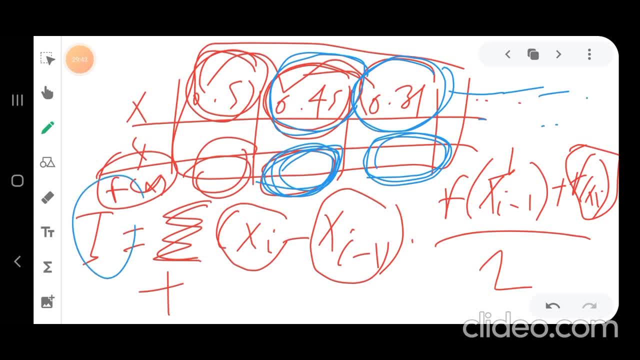 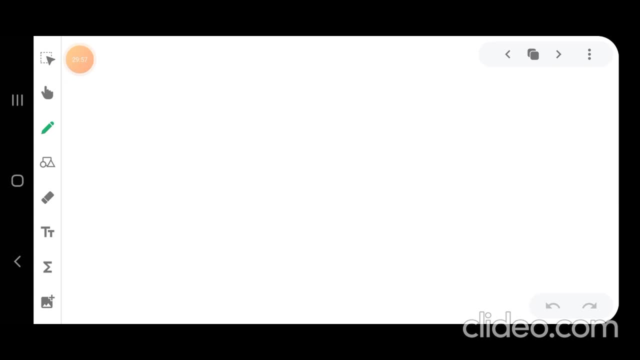 this is your integration. you can use this equation if you have unequal intervals. it's just a numerical equation, okay now. so that's all. that's all for the simple batch distillation. now let's discuss the rectification, and we are going to discuss only the binary. 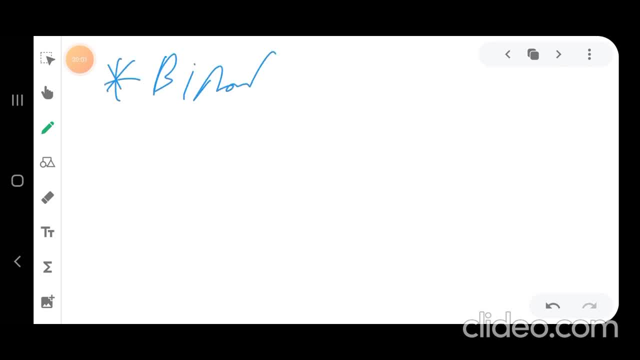 binary mixture. i want to start with simple things, so we'll discuss binary batch rectification. binary means we have only a and b. suppose in the a it is no more volatile and b is the heavy. as we said, we have two modes of binary batch with this rectification. the first mode is constant r. 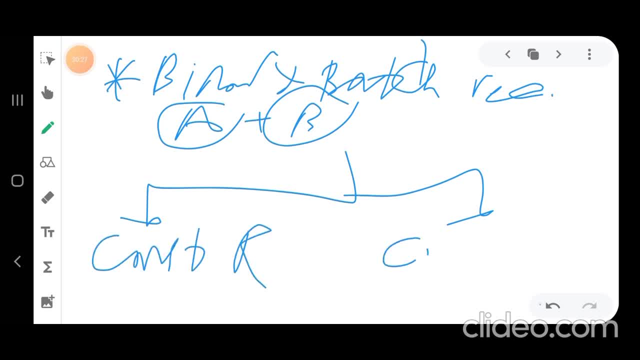 the second mode is constant d or constant xd, so let's start with them. and, as we mentioned, it is easier to work with constant r from the control process point of view than working with constant xd, so let's start with the easiest one, which is constant r. 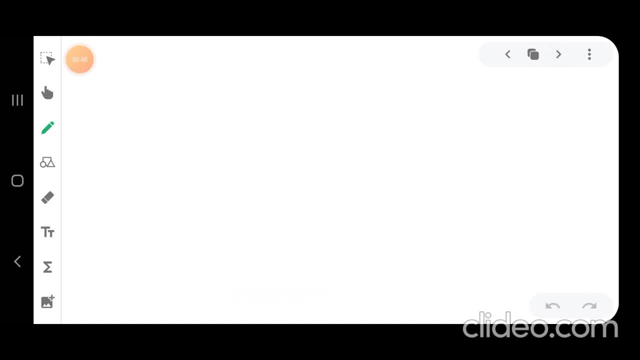 what we have to do here for constant r, batch rectification. so we will start with constant r. this is for constant r, this is for constant r, and we are going to do some assumption here that we have a constant boil up. what do you mean by boil up? again, you have here, this is your, still both, but now it is rectified. 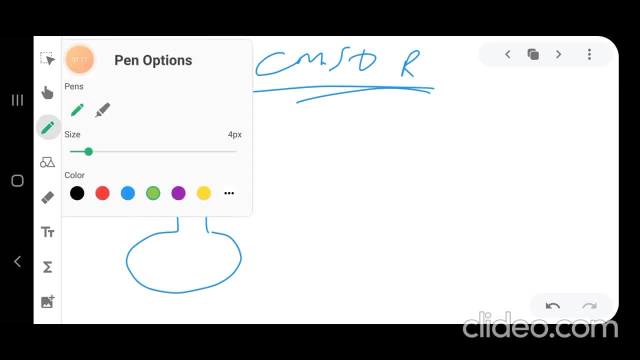 rectified means we have here some stages. then you take this. so, in order to maintain a constant contact between liquid and vapor in these stages, you need to draw some reflux back and then you take your product. so this will be your product. you collect it on a tank or whatever. okay, so. 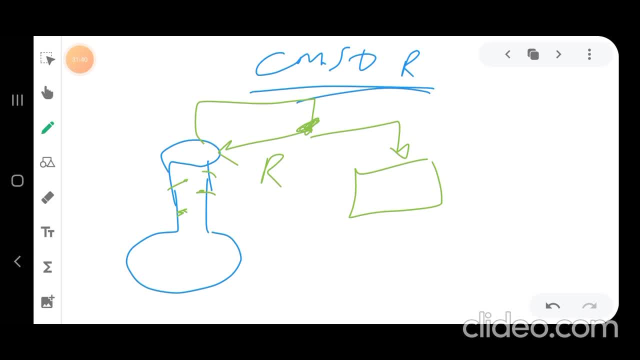 we are going to assume that. we are going to assume that this vapor is leaving the system. let's call it v, which they call that boil up, boil up. we are going to assume it constant. we are going to assume it constant, and you know that r is constant for this type. 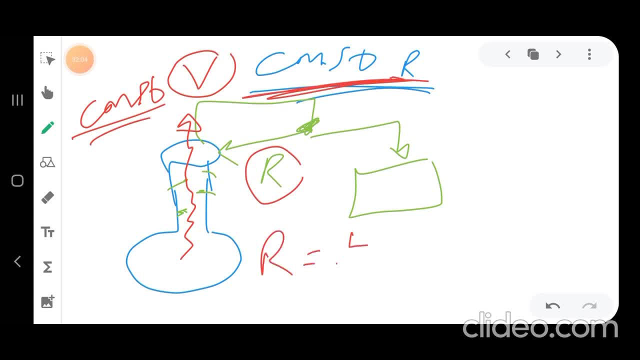 and r is just l over d right, this d distillate and this is the l, the liquid returning to the still both. so if you have a and you know that, from material balance that v is equal to d plus l. so what I want to say here is, if you have constant v and you have constant r in other, 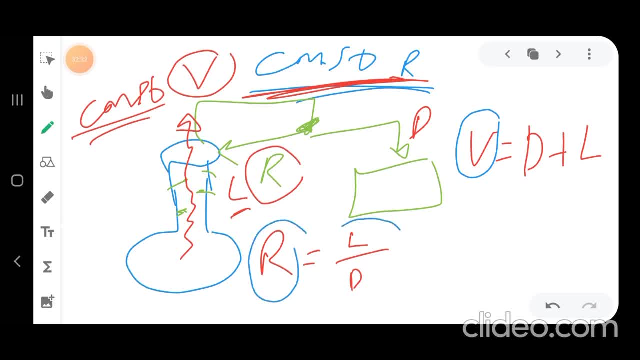 words, you have constant l over d, so l will be r multiplied by d. so this r by d will be constant, so you will have also constant l, so for sure, you will have constant d, so everything here is constant. in this case, you can find the time needed for distillation, as we mentioned, using this equation: 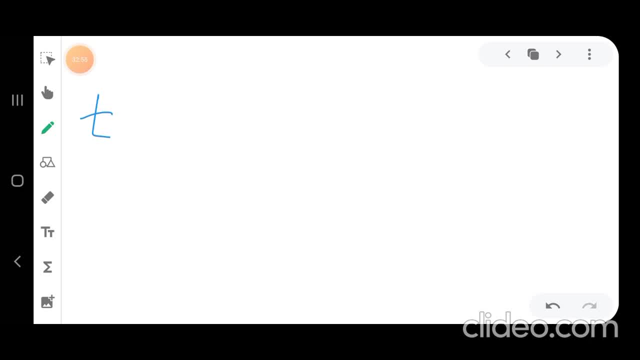 time will be w naught minus w over d. then we can play with this equation. we can say in w minus w, naught minus w, and this d from material balance is v minus l. right, if we rearrange this equation it will be v minus l. so we can say that v minus l is equal to v minus l and v minus l is equal to. 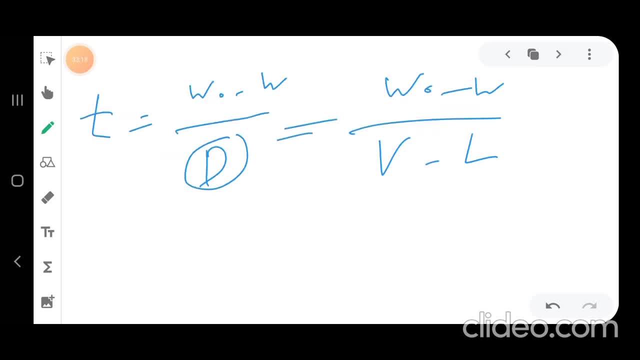 okay. and you can further play with this equation by defining the reflux ratio. you know reflux ratio is l over d, okay, a flux ratio, l over d- okay. so for example, you can divide both sides by d or manipulate this equation somehow at the end of the equation. so we got d over first until sente zas equals equal to d over d. so we know that. 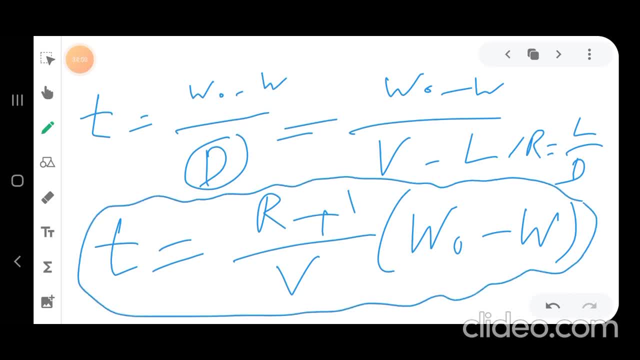 then if we have this equation, we also have a Фp left over in summer, the value of this equation. so we want to stay at the start point to calculate the time of the distillation. now, what if we לקveer då? ordinarily you will reach this equation, which is: T is equal r plus one over the w, naught minus w. so this equation can be used, if you have a constant r by distillation, in order to calculate. 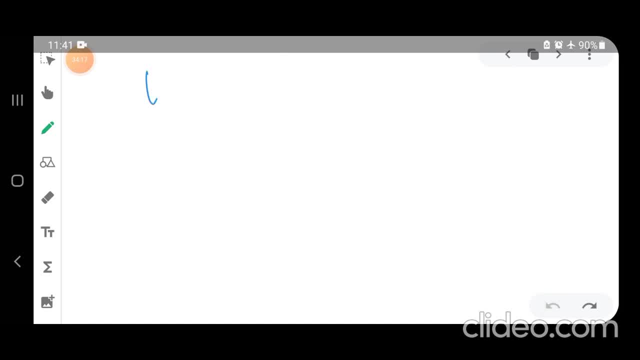 interested to calculate the w, the quantity that we left with and still brought after the distillation. again, we need to go back and use Rayleigh equation, this equation. if you remember this Rayleigh equation, yeah, I think, let me write it again. yeah, we need Rayleigh equation, which is length w over w0 as equal to integration from xw0 to xw. 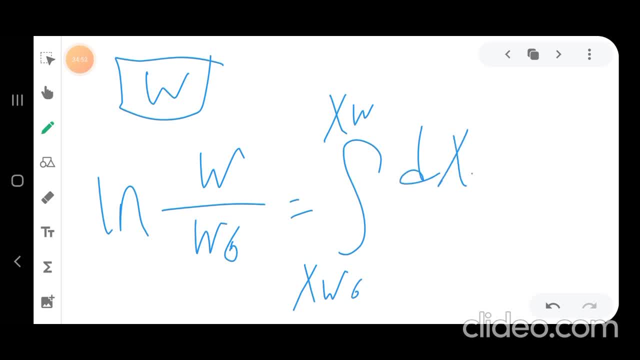 dxw over yd minus xw. you need to. so again, let us call this one. let us call it i. okay, so again, w will be w0, e to the power i. the problem here is how to calculate this i. so if we know this i, we can use this equation directly to get w right. 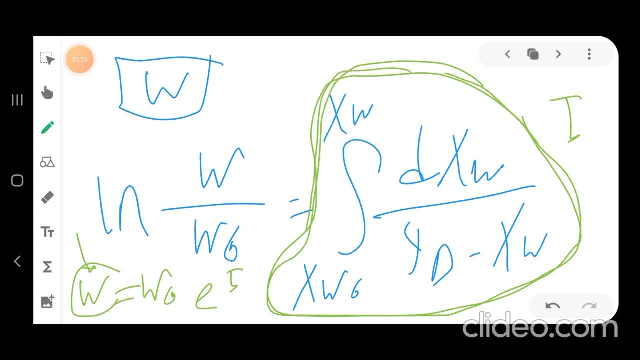 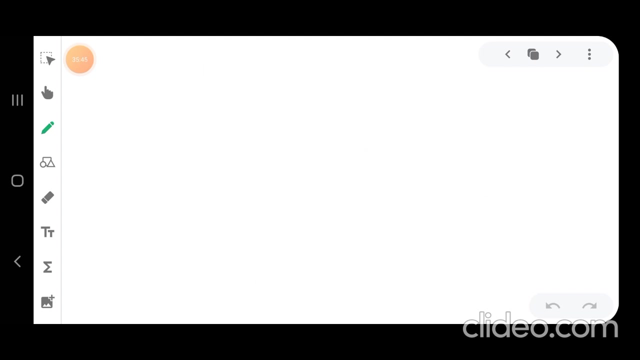 so this is again an integration, again we are going to use, we are going to use, we are going to use the numerical integration in order to integrate this and how we are going to do this. we need, first thing, is to plot. we need to plot like this: see, you need to have 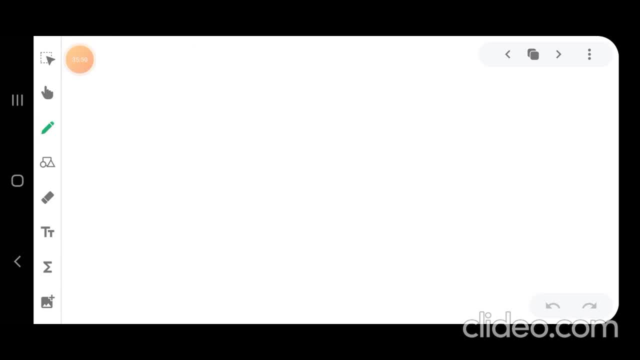 your suppose this is your graph paper. this is your graph paper, okay, and this is your x and this is your y: liquid and vapor compositions, and this is your 45 degree line. let's say: this is, yourhoo, your equilibrium curve. okay, again, this is constant r. and when you say constant r, this: 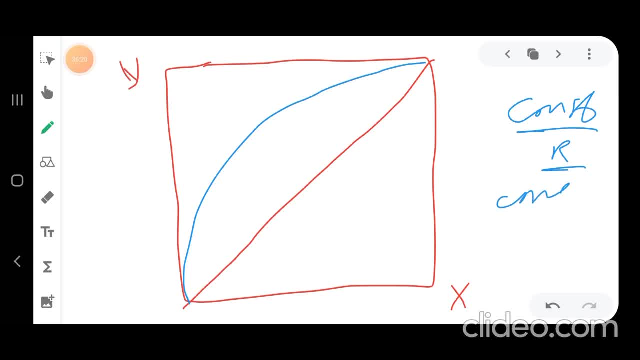 means constant slope. slope will not change and xd will change, so you can start at time 0, this is will be your xd, which is xd0 at time 0. okay, then, using the constant reflux that you know, you can calculate the slope. right, you can calculate the slope and from: 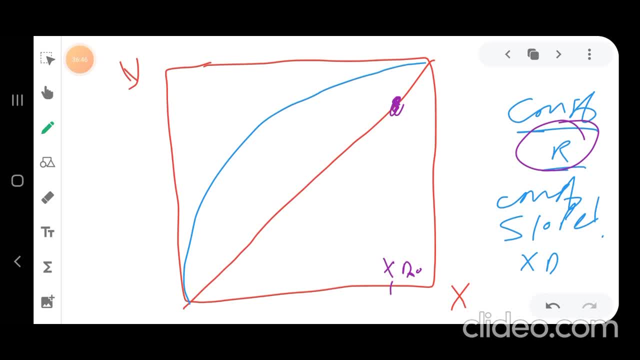 a slope and the point: you can draw a curve, okay. so you can draw a curve like this, okay. and suppose let's say we have a curve like this, okay. and suppose let's say we have a curve like this, okay. and suppose two stages, let's say we have a two stages, for example- then what you will do? you will. 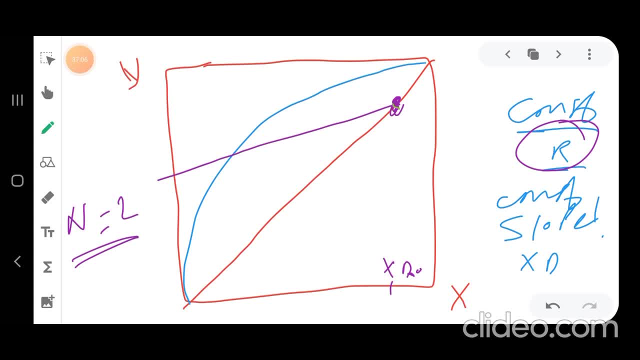 start from. as makeup delay method, you start from xd0, then you go one, two, so this will be your xw0 at time 0 at xd0. okay, then we need to move this line again and again, we move this line. it is constant, also the same slope. so 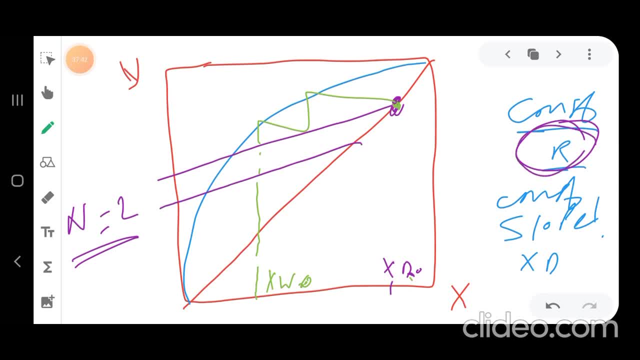 so all lines will be parallel. we need to move this line. but the question here: where to stop? until where we stop moving this line? we stop until a point. we stop until the point that if you draw this number of stages, you will end up with x, w, the final. after some time, the final. 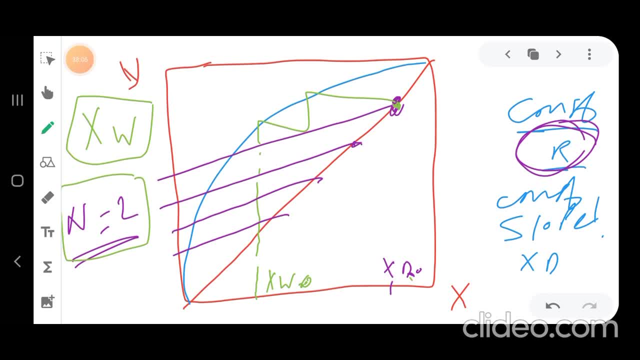 composition of the mobile trial component and the still pot. so it is like you will stop here where you have. you draw these two stages, then the value here will be x- w- okay. so the first step is. the first step is to draw this line that starts at x- d- naught okay, and x- w- naught. 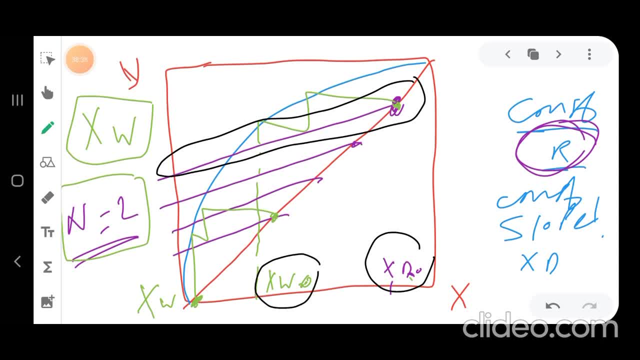 then you draw this line, that's this line. if you draw it and draw the stages, you will end up at x w, which again refers to x d. then in between, we just draw some random line. for example, let's say three lines, one, two, three. you draw this random lines. okay, why we are doing this random? 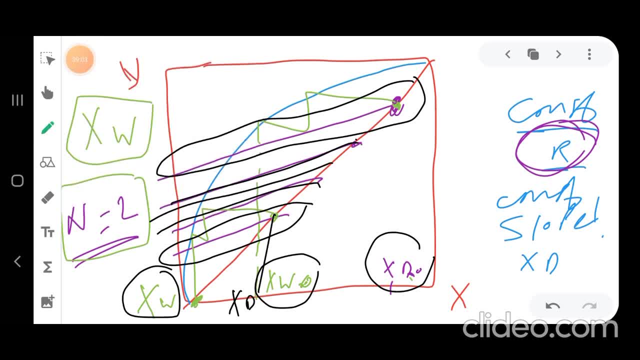 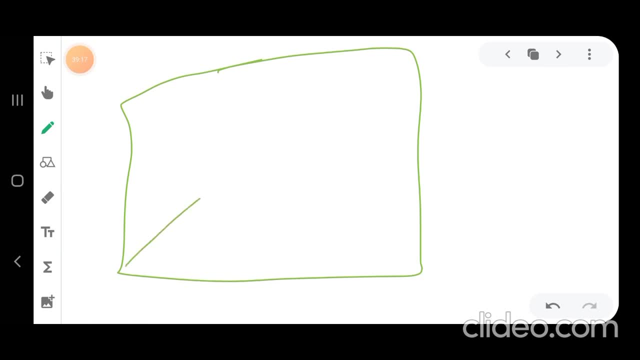 lines because we will need them in integration. so you do this random line, then you start counting two stages, then you read x, w, so it gets crowded here. let me write it in simplified way. so what will happen that you will get? you will get different values of 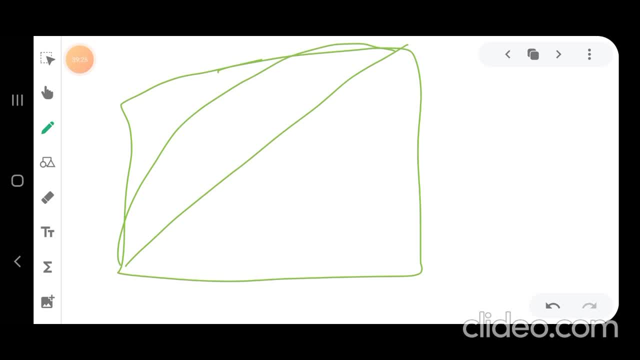 x x, you will get different values of x d and different values of x w. so let's say you get starting from. you get x w, naught from curve one, then x w, one from curve two, then x w, two from curve three, x w four, three from curve four, all the way to x w, which is the final composition. and at 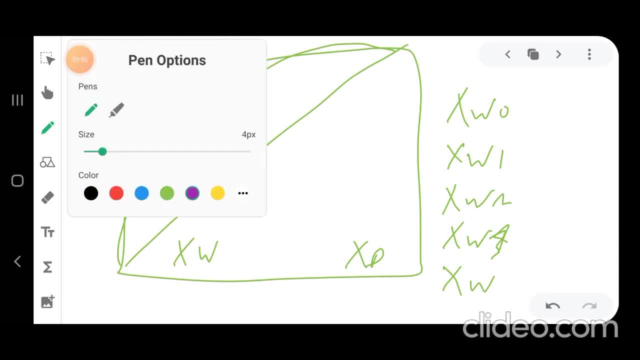 each. at each x, w, you get the corresponding xd, xd, naught, then x, xd1, then xd2, then xd3, then xd, the final composition. okay, so these all you can read from the figure using the given number of stages. okay, then what you will do is that. 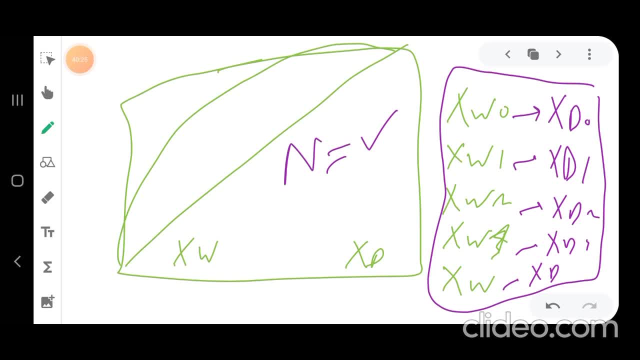 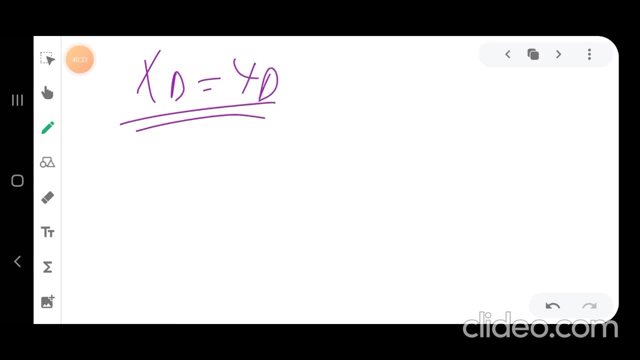 you will go and of course, xd is same as yd. we are assuming a total condenser. okay, so xd same as yd. so what you will do, you will draw a table to integrate numerically then this table. you will start with x w, starting from x w, naught you all the way until x w. okay, then you write the corresponding xd or yd values. 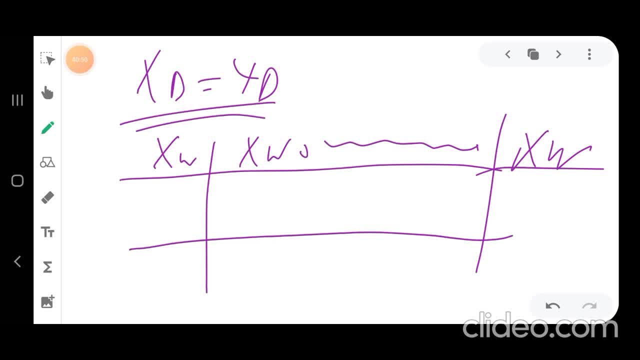 then you write the corresponding xd or yd values. then you write the corresponding xd or yd values. they are the same- that you again get it from the figure xd naught all the way until xd. then what do you want to integrate? you want to integrate one over yd minus x w. 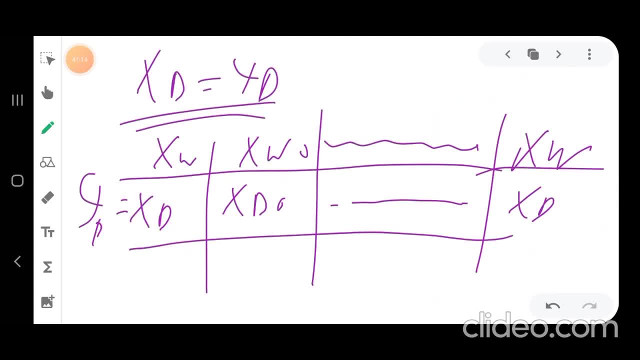 then what you will do? you will find f of x, which is one over xd minus xw, so you will find these values. this value, then the total YU value opinion, is 1 over xd to the y wave. then what will you do? you will find f of x, which is one over xd minus xw, so you will find these values. 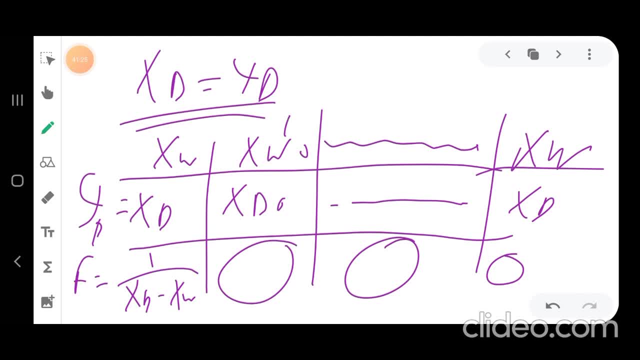 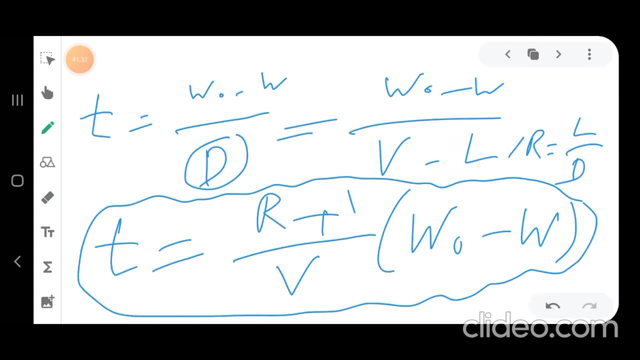 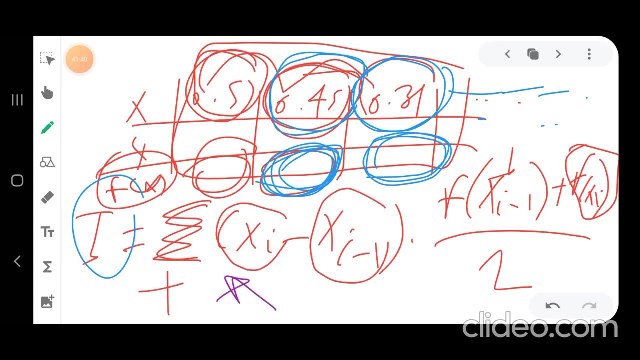 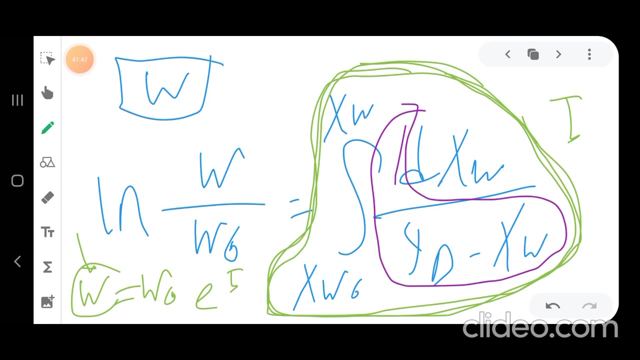 you see, in most cases you will have unequal intervals. so, what you need to use, you need to use the trapezoidal rule based on unequal intervals, this one, this trapezoidal rule based on unequal intervals, in order to integrate. then, once you integrate, you can get the integral. from the integral you can get. 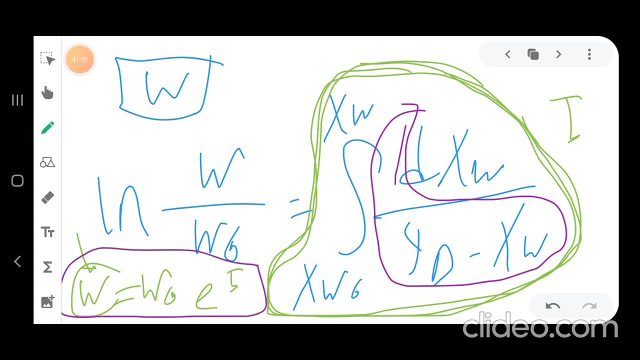 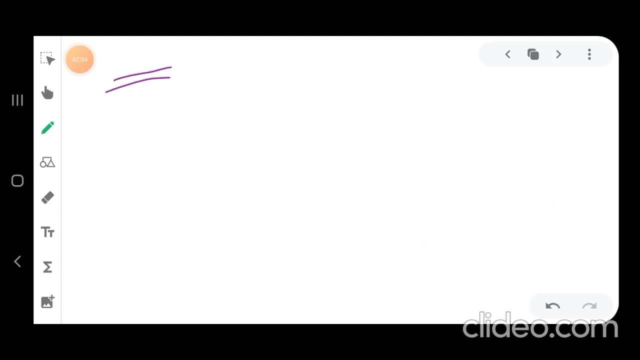 from the integral exponential of the integral w0, you can get your w. so that's it. this is for the batch rectification with constant R. the last thing here is what if we have a constant XD, batch rectification with constant XD, since this XD is constant, we can do a very good, a very good. 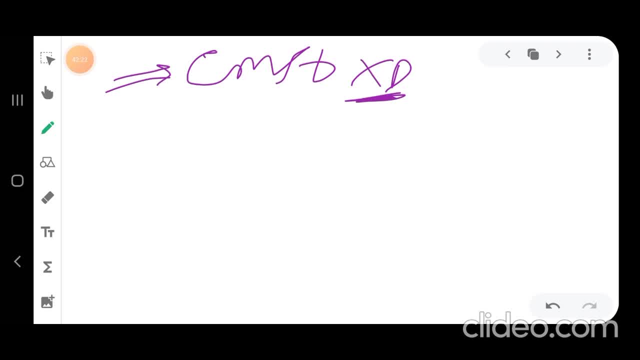 assumption that is highly valid, that we can see the instantaneous composition of D is equal to the average composition that we are going to collect at the end of the day, because XD is constant, it will not change. so this is a very good assumption that we can do in order to solve this type of problems. but again, the problem. 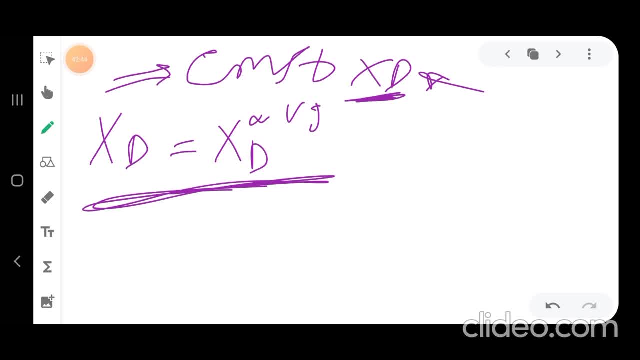 here is that again we are going to assume constant, boil up constant V and but the problem here we have this reflex ratio. it is not constant and you know that this R is L over D, so this one is not constant. so L over D or L and D, each one of the L of D will be variables, would be not. 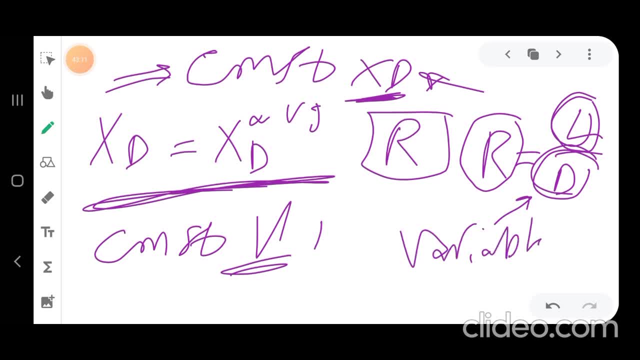 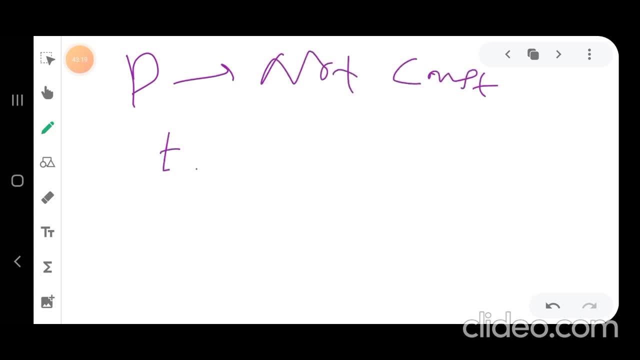 constant. in other words, D is not constant, so you cannot use. D is not constant, so you cannot use this equation w0 minus W over D. no, because D is not constant, which is because you are going to eliminating this equation. after you have got rs airplanes, you can use each one of them all the way around, so not. because we can use this paper. so this is right now we are videos, which the three will be chosen at the time of your listening to my lecture shouldkovs, so that you memorize each one, because I want to тради Tatso, because thisламain1502, this is ц- deutschen, because z is nothing, ed gin. 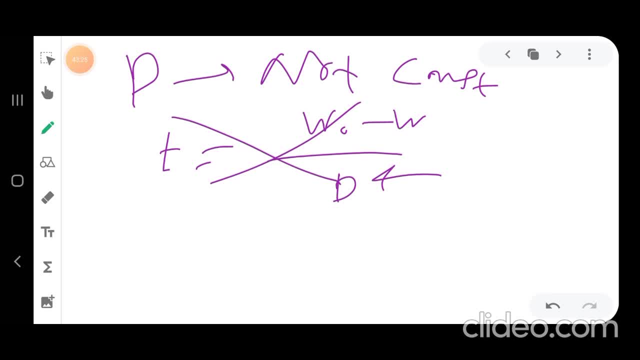 and so we will try to retrieve here. we need to Shanghai zone and we should not constant what we need to use. we need to apply an equation to calculate the time. we need to apply an equation, rather than this equation, that helps us to calculate the required time, and this 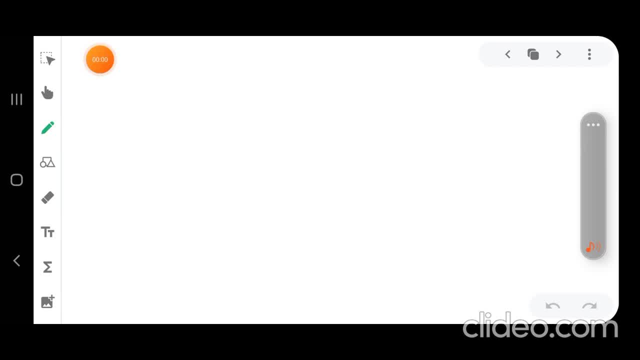 times. okay. so since, as we said, D is not constant, this is not constant, so we need another equation to calculate the time. we can calculate the time. so this integral equation where we have w0, X'd minus X, w0 over V, integral from xw to xw0, it's a reversed integration from n to 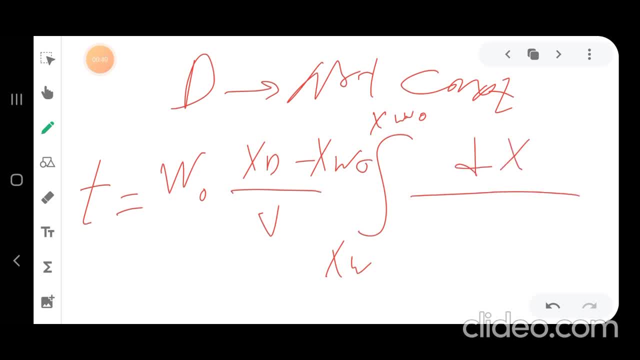 beginning: dxw, 1 minus L, over V, xd minus xw, whole square. so let's go over this equation. 10 by 10. what's this? w0 is the initial quantity of liquid in the still-pot. what's this? xd? it's constant, constant xd. then it will be the 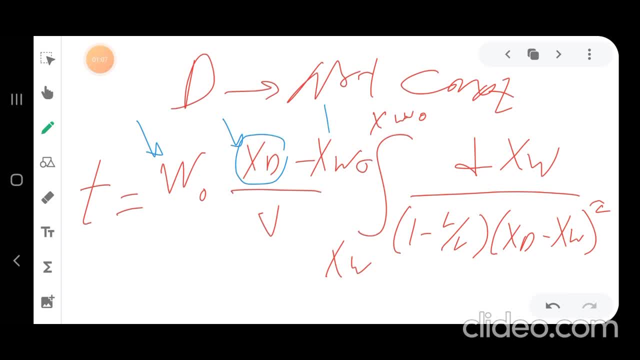 constant district composition that we have. xw0 is the composition of the more volatile component in the still-pot. initially, V is the vapor boil up, boil up rate, okay, and xw is the final composition in the still-pot of the more volatile component, xw0, as we said, the composition of the more volatile component in the still-pot. 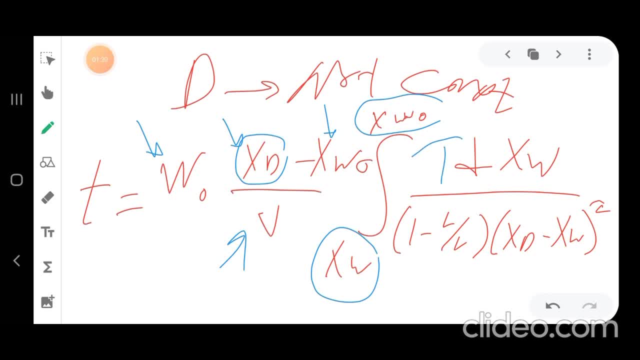 then we have: this is our integration. we are integrating this function with respect to xw. so this is our f, that we are going to integrate. so, again, we can call this part as a whole, we can call this part as I, as we said before. then, if we find I, we can multiply it by: 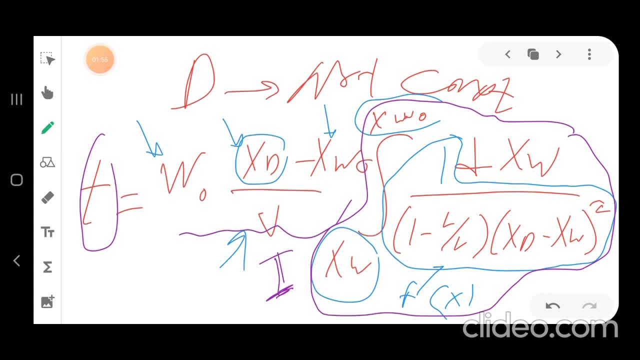 this term to get the time okay. so in this I you can see if the first thing that we have here we have L over V. what's this L over V? it is like make a telly. what's this L over V? it is the slope. it is the slope, so you can calculate it. 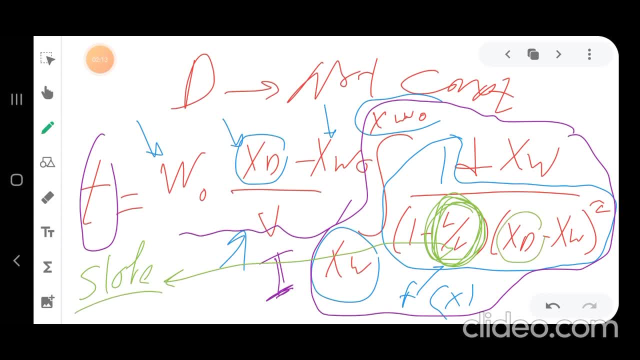 from the slope of the line. okay, and again, xd is constant, which is the composition and the distillate of the more volatile component, and xw is a variable because you are integrating with respect to Xw, dxw, so this Xw will be variable. the question here is how to determine this slope and xw. then you can. 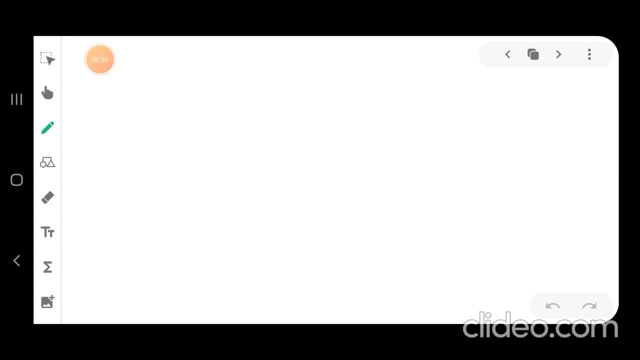 integrate it. so you need to make a kind of table. you need to make a kind of table like this to numerically integrate this integral. we want to find I this integral to get the time so we can make a table like you: start with your independent variable, which is, in this case, your. 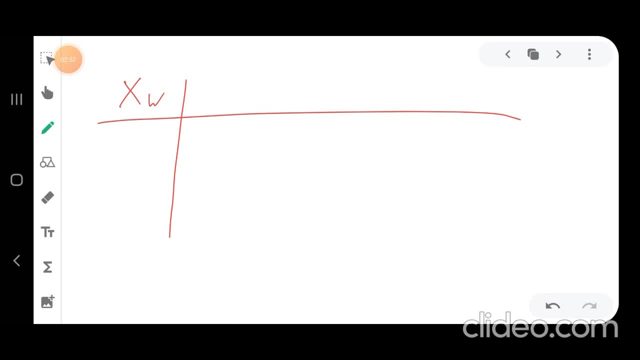 independent variable XW. then you give the slope L over V, then you find f of X. okay, and what's this f? this function that you have, that you are integrating, is 1 minus L over V, multiplied by X, D minus XW, whole squared. okay, so you will. 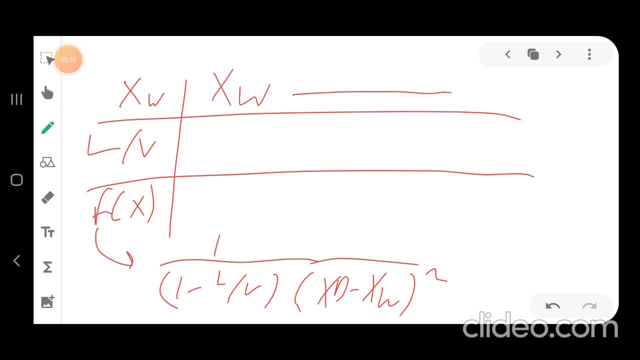 start the values of XW, starting from XW up to XW naught. you will have different values then L over. but the question here how to get this XW on the slope again you need to draw using make a delay. so suppose this is your graph paper. this is your graph paper and this is 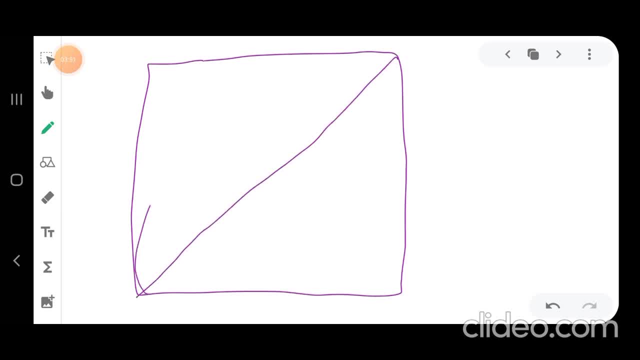 your 45 degree line and this is your equilibrium curve. so what you will do? you will specify where is your XD. so this is X and this is Y here, for example, here is your XD, so XD is constant and we have variable R. this R is variable. 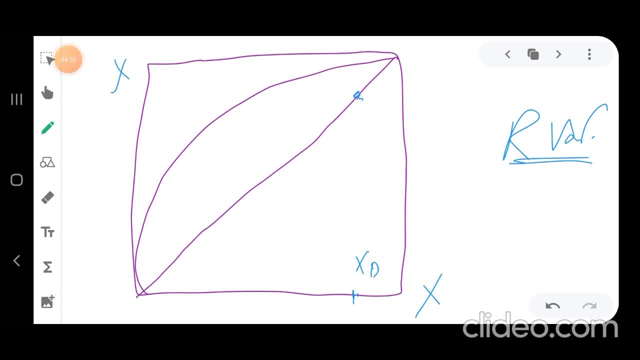 right, and we are in the case of the constant XD, so variable R, so the slope will be variable. this is slope will be variable. okay, so you need to start with a 9. that suppose, again, we have two stages, or whatever stages you have. suppose we have two, so you need to. 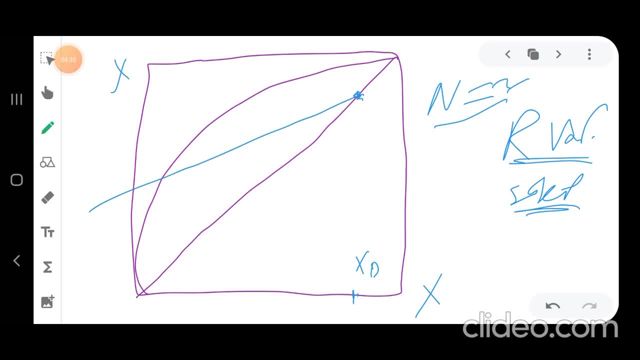 start with an initial slope that if you draw this slope then you count the stages as two. then you will end up with XW naught initially. then you need to to draw another curve. you need to play with the slope and play, play with the slope of the curve starting from XD until you draw a slope, that is, if you 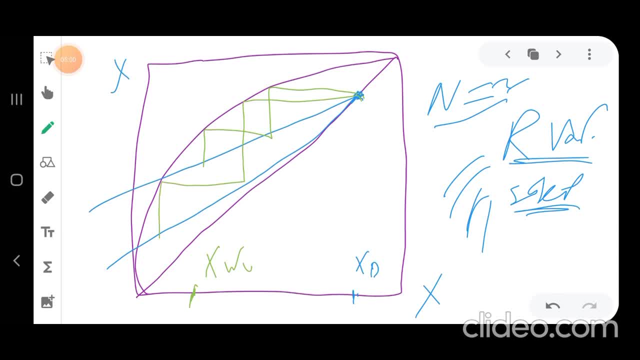 start here and you count the stages. two stages, you will end up with XW. you need to satisfy this criteria. okay, then, once you have these two lines, you can take, for example, two lines in between or four lines. as more lines you take, they more accurate answer you get. 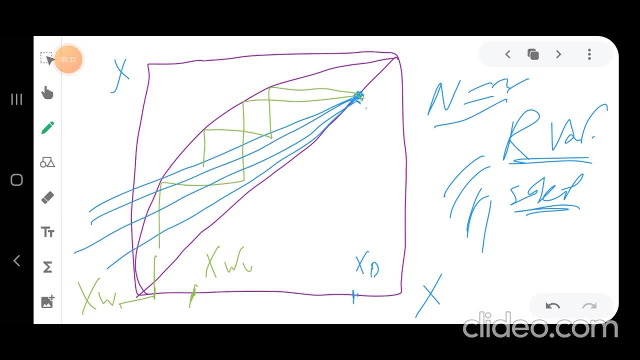 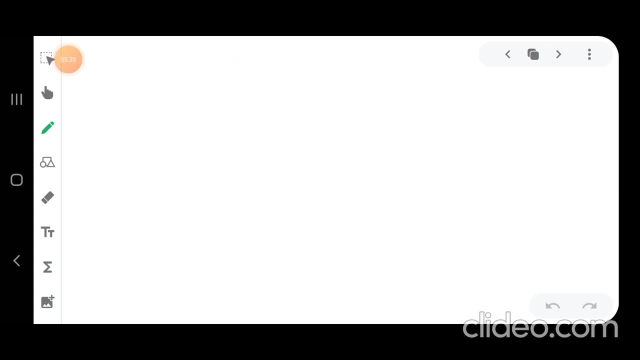 and that is a numerical integration. okay, more points, better answer. okay then, for each line again, you will do the same story. you do the same story. you count the number of stages. you see you need XW for each line as a summary for each line. for each line. for each line, you will have different. 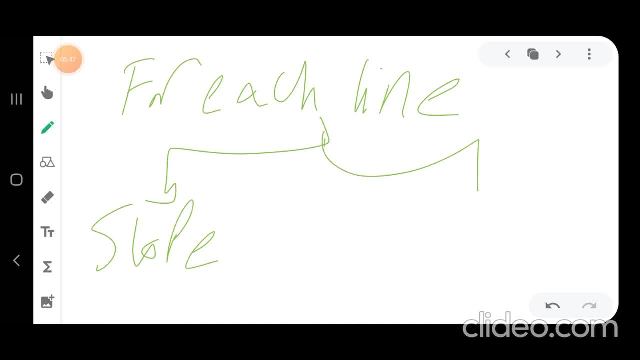 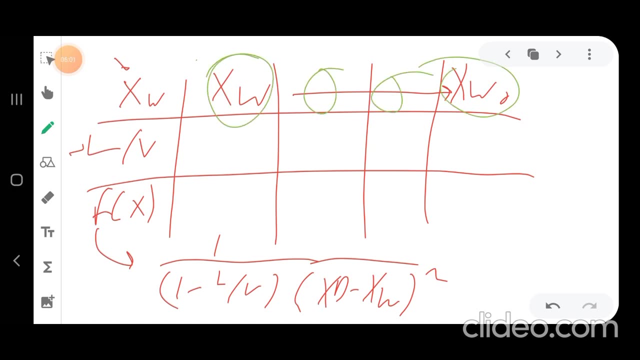 slope, of course, and you will have different xw, okay, for each line. so you will take these values of xw and the slope. you put them here. these are different values of xw, starting from xw to xw, not y, because the integration is from xw to xw, not so. that's why we start from xw, all the 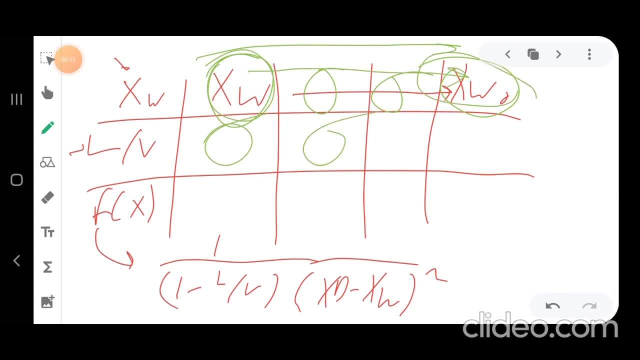 way to xw not. then you plug the values of the slope that you have. the slope is l over v, as we agreed before. then you calculate this f of x, knowing the slope and xw, and you have already constant xd. you can get different values of f of x. 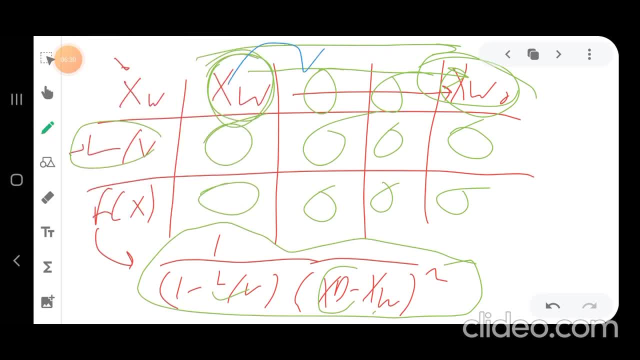 and again, it is very difficult to have equal intervals here. it is very difficult. that's why you usually you need to use the trapezoidal rule, based on unequal intervals, to integrate it numerically. as we discussed the trapezoidal rule, it's the summation of: 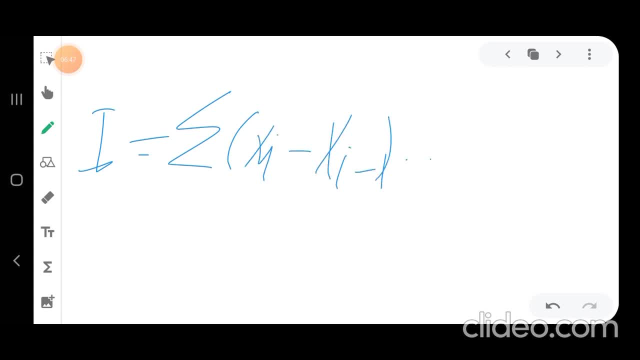 x i minus x. i minus 1. multiply by f of x i minus 1 plus f of x i. multiply over 2. so it is like this: one is the average value of the function. multiply by the interval, then you take the summation for all. 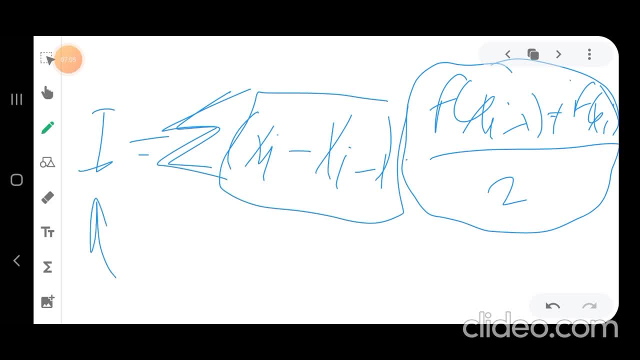 points. that's it. you can take the integral. from the integral, you can get what, you can get the time required, okay. now what about w, if you are interested to get the final amount that you left in the still part of the distillation finishes? okay, so how to get this? the easiest way? 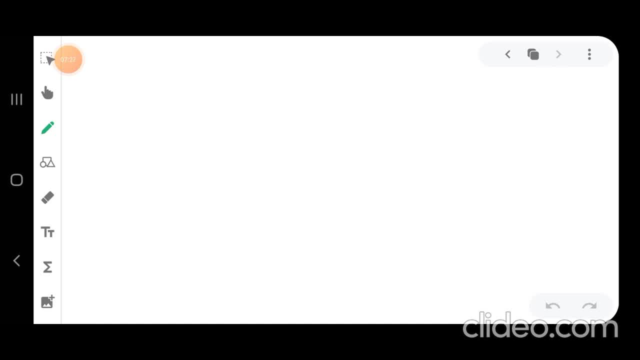 is to apply the equation that we derived it before for the material balance, which is this equation. this is the easiest way. no need to use the release equation and waste your time and integrate and you will get same answer, of course, or somehow closed answer, but the easiest way is to apply this equation you need. 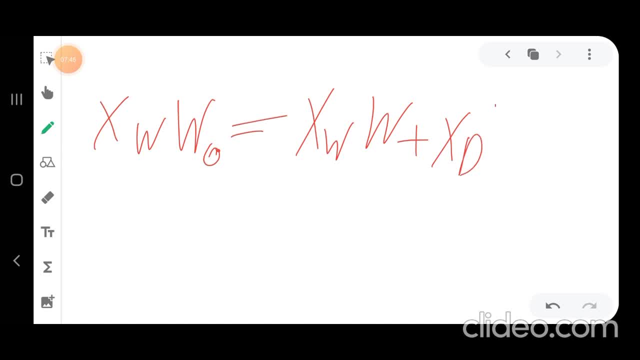 to apply this equation. you know the material balance equation around the still pot. so we derive with these two equations, if you remember this first equation and the second equation, as w naught is equal to w plus d total total, if you rearrange it you will get D: total is equal to W naught minus W. okay, so we. 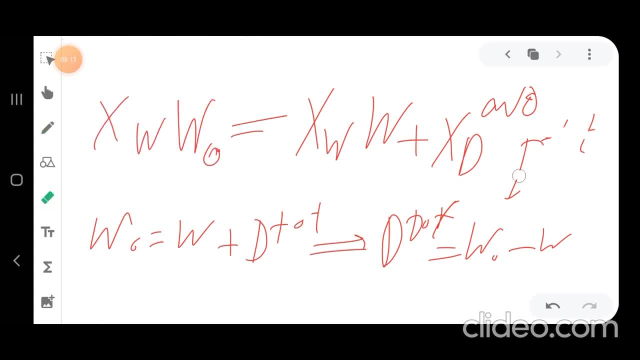 can, we can remove this D total here from this equation and then instead of it you can write what you can write: W naught minus W. okay, then you will see what's the only unknown here. we know XW, our final composition that we want to achieve in this third part. for more volatile component. we know W, naught, our.